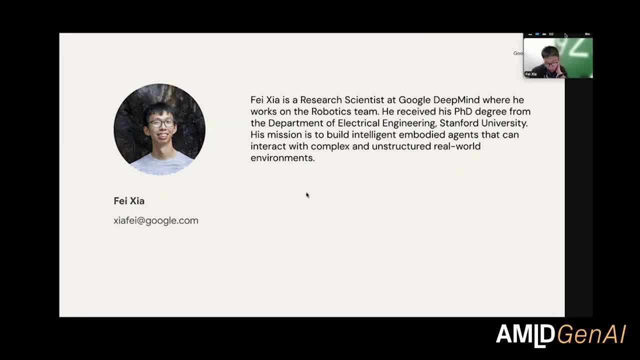 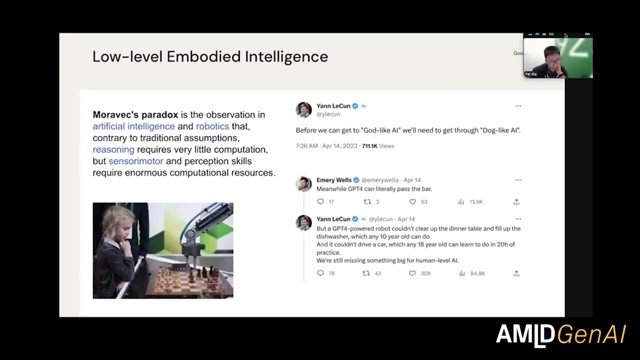 embodied intelligence, embodied perception, and our mission is to build intelligent, embodied agents that can interact with the complex and unstructured real-world environments, such as human homes, Right. so in the what is embodied intelligence? It means an agent that is intelligent and generally physically capable, that can interact with the complex world. So for a long time, there is more. 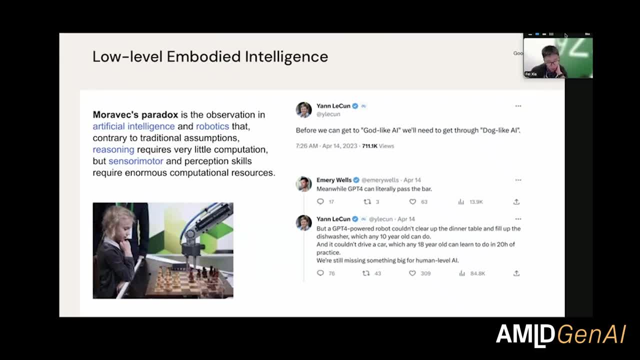 of this paradox. More of this paradox is an observation that is in artificial intelligence and robotics, that the easy problems are hard and the seemingly hard problems are easy. So, for example, you can have the AI be the test champion of human, but you still need someone to move the. 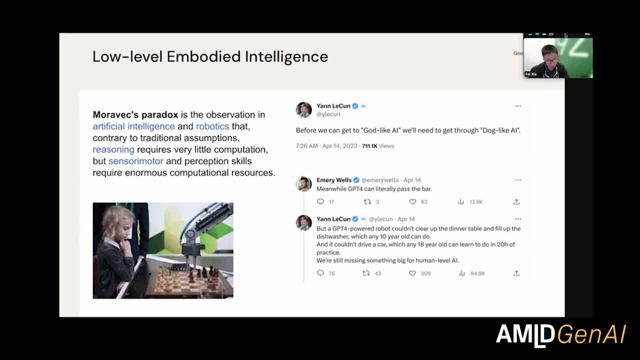 test piece right. so the physical capability of the robots are not still not there yet And robots testing in the last three or four decades has been relatively slow, although a lot of the progress has been made, But still we don't have our own robots yet. So we think the foundation 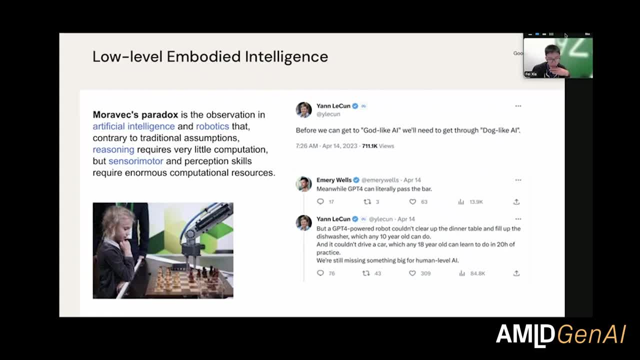 model might be able to change that. Another observation is the other convention: before we can get to God like AI, we need to go through dog like AI. So what is a dog like AI? It's an AI that is generally capable in the environment. it can work with your computer, it can walk and it can. 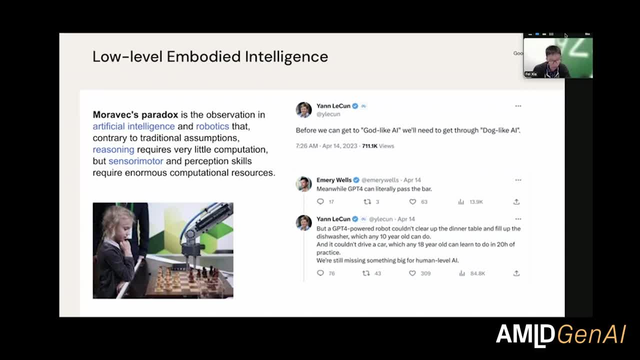 work with your laptop, you know, And we have to think about the environment that we live in, right now around and it can grab things for you. Some argue GBT-4 might already be able to do this. However, Yelatan argued that there should be more power for a lot of people to swing out the dinner table. 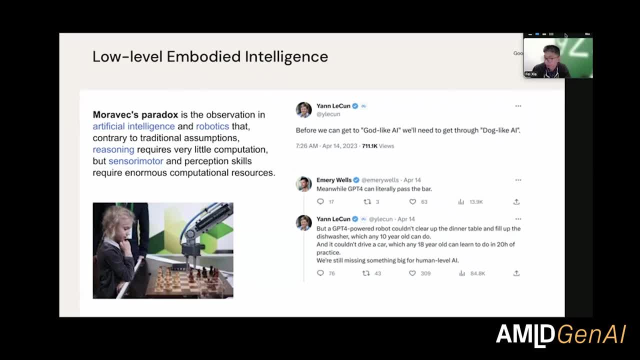 and fill out the dishwasher, which a 20-year-old can do. And also there is a problem on sample efficiency, like the consumer can learn to drive within 20 hours of practice, while AI needs to build a huge amount of data. So we don't have the dog-like AI yet. 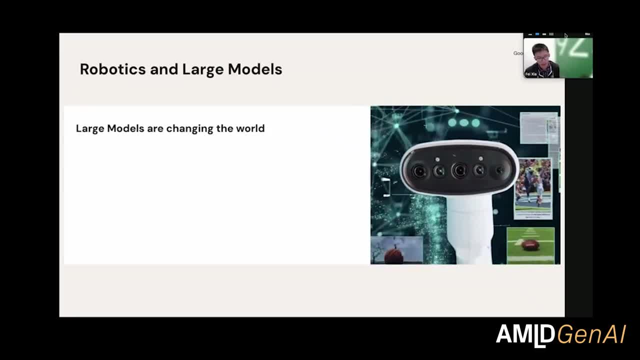 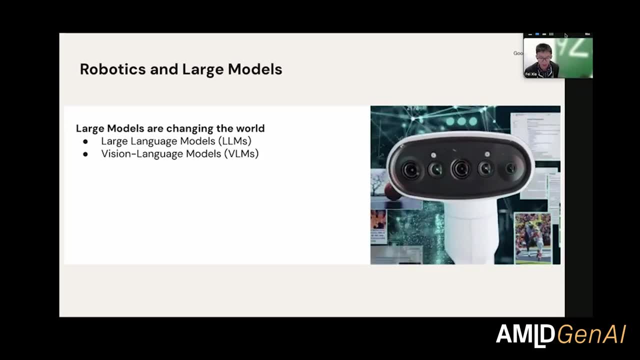 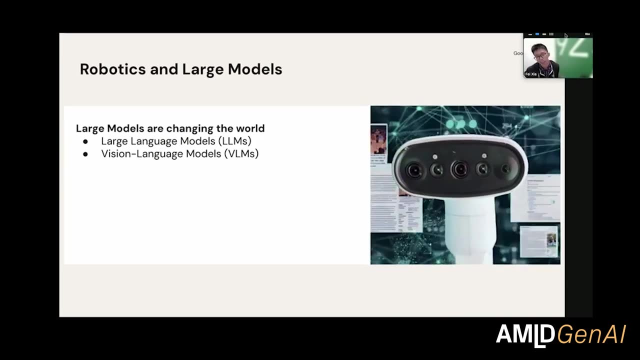 So most recently, language models are changing the world. There are language models that can explain jokes. they can have a good conversation with you. they can help you write emails and everything. There are also visual language models that can understand the environment. You can ask. 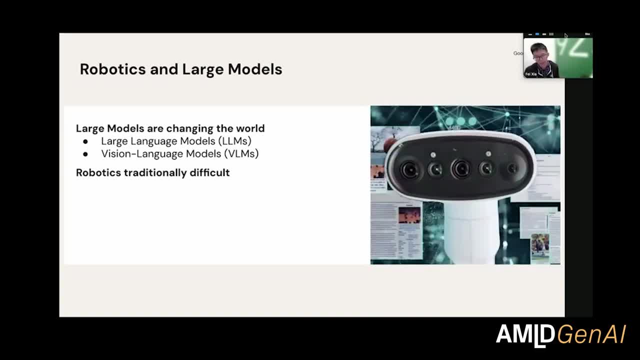 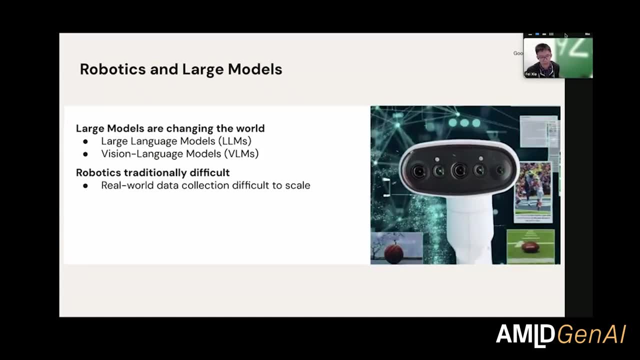 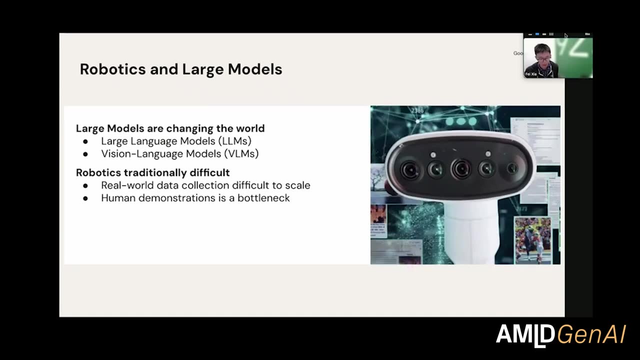 questions about an image. you can ask it to caption an image for you and do all sorts of neat things. However, robotics are traditionally difficult because real-world data collection is difficult to scale. That's also the motivation for this why we use simulators And human 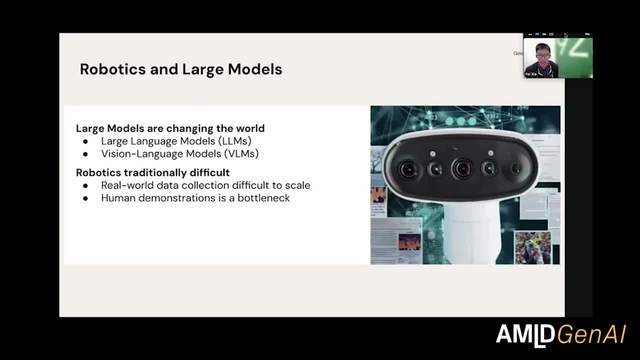 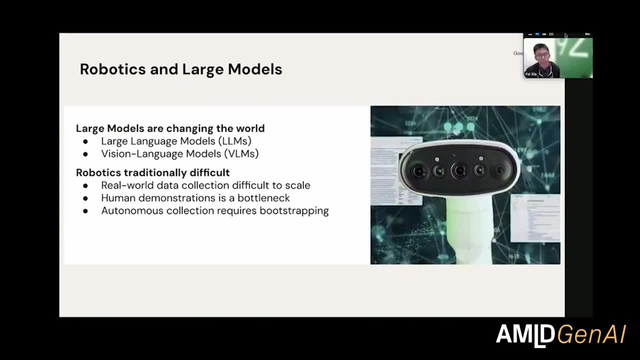 demonstration is also a bottleneck So it's hard to come. So robotics, data are hard to come along And autonomous data collection requires a lot of effort and some have to be done in different teams and it requires a lot of bootstrapping. 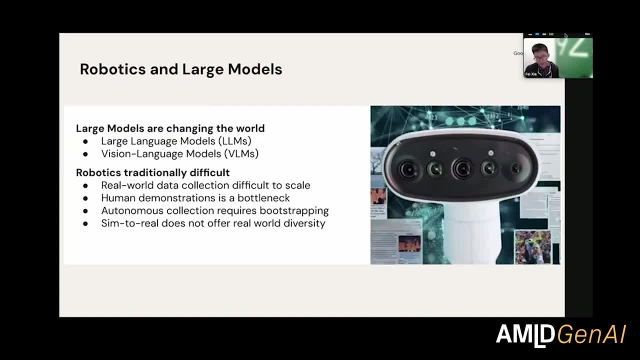 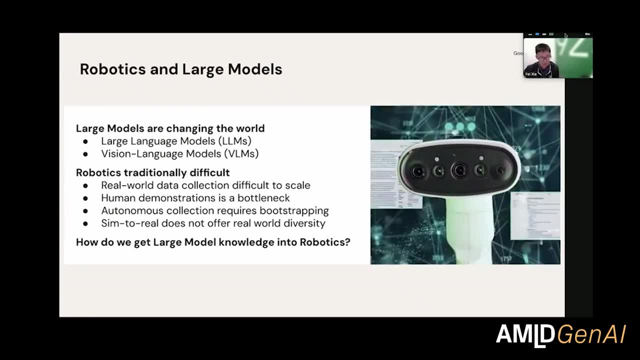 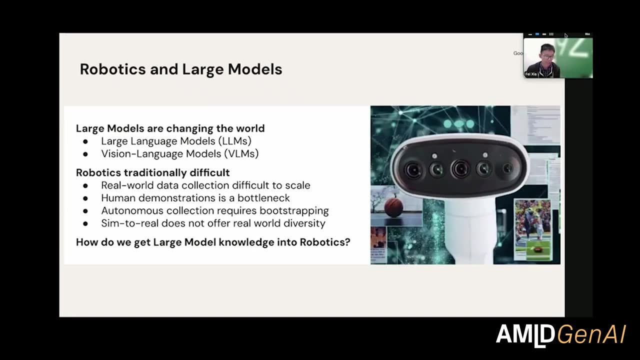 And Sim2Real does not offer real diversity, And Sim2Real is also an open problem. There's no agreed-upon solution for Sim2Real. We are thinking about using large language models to provide more knowledge, provide semantic knowledge of the environment and use them in robotics. 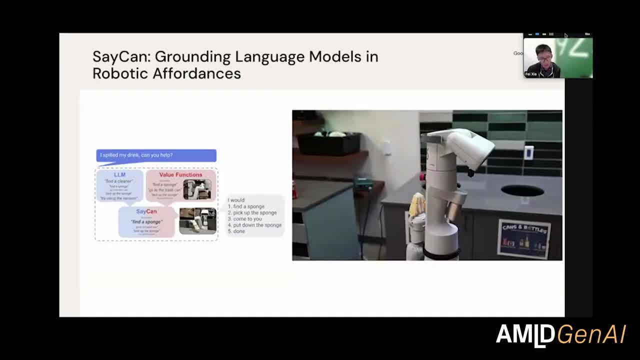 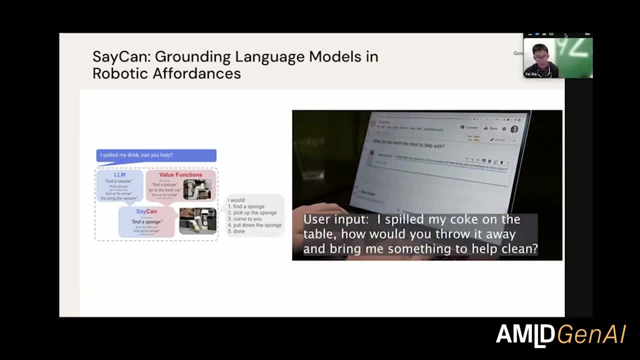 We can try to get the large language model knowledge into robotics. How it works, I'm sure in this line of work, is called SATAN. So SATAN is a large language model for robotic performances. So the insight is that language model can hallucinate. 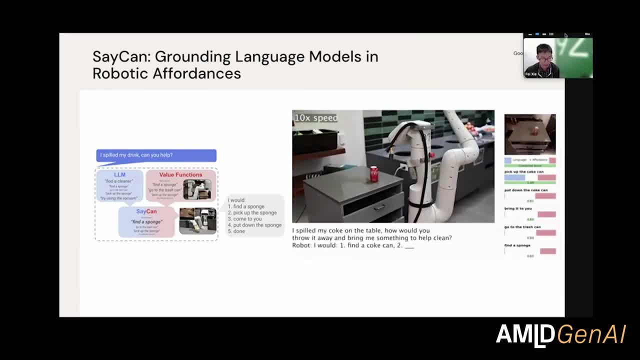 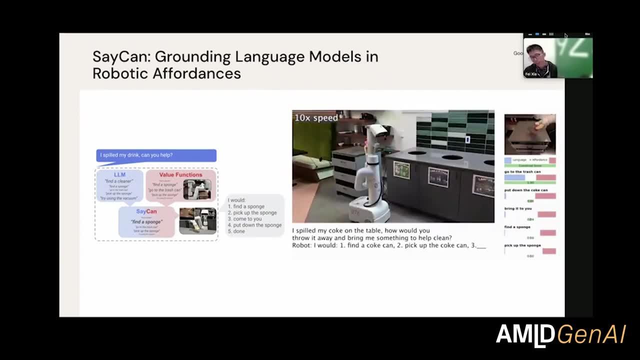 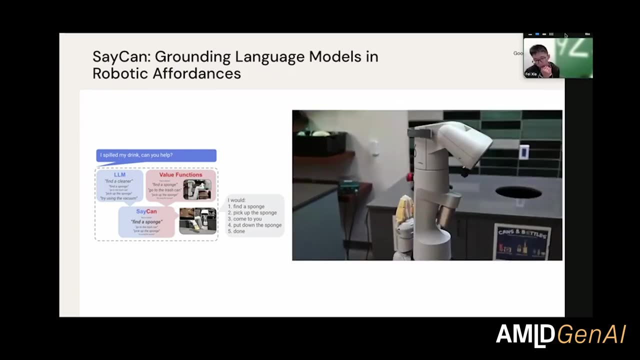 but you can ground them in robotic performances. So language model tell you what to eat And there is a separate module for performance that tell you what you can do here. So let me just play this jit. So in the jit there is a unique model. 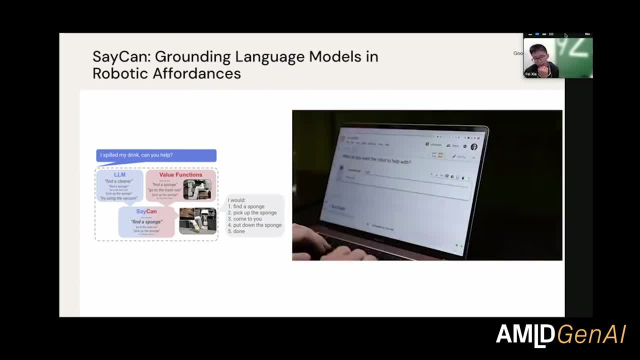 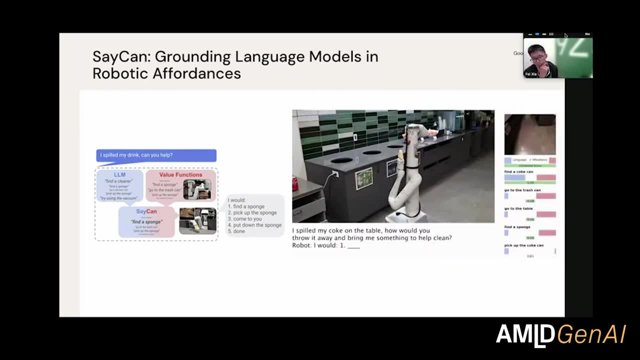 where the user asks the robot a question. I steal my food On the table. probably you throw it away. I'm going to eat something to help clean. And then there is a language model doing the planning for the robot. The language model is the brain of the robot. 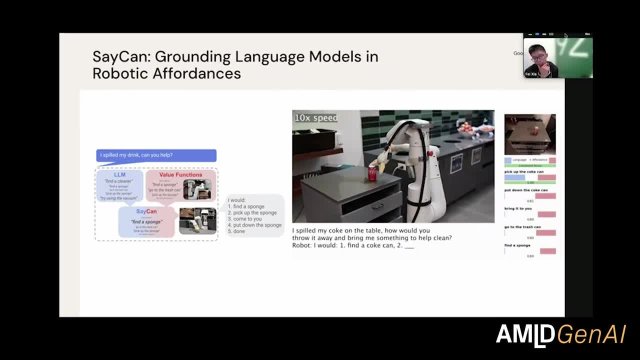 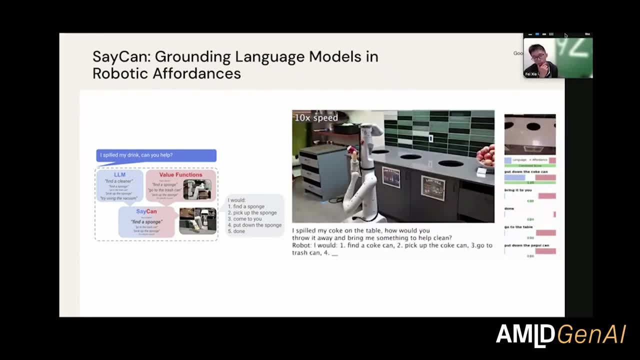 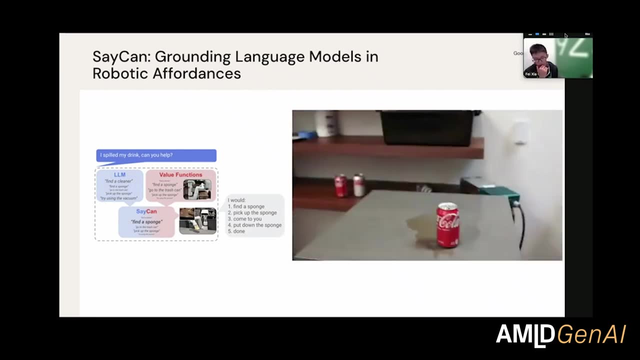 And there is a function serving as the eye of the robot. It's deciding what the robot can do in a certain spot. And there is the manipulation policy serving as hands of the robot, Right Hands of the language model. So the planning module helps you find a hole. 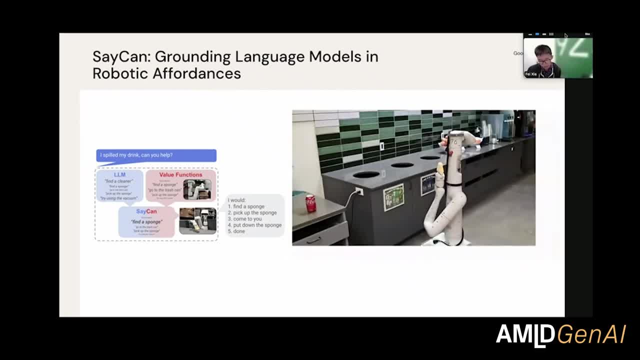 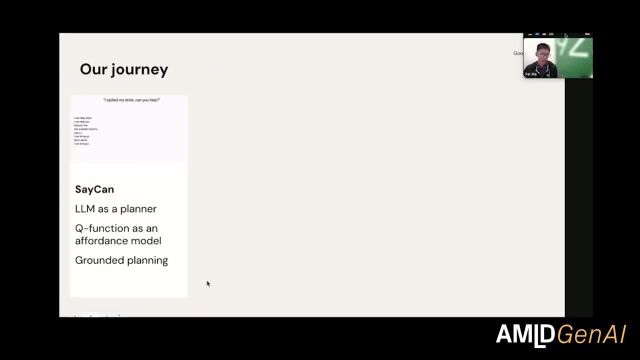 and throw a hole there and later bring you a sponge. So this is our first adventure in using that model in robotics. We have been through quite a journey, So first we used language model as a planet And we used Q function as a model. 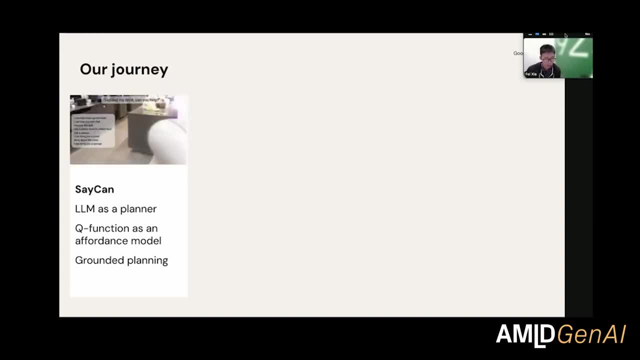 to ground the language model and do some grounded planning, Then we essentially find The loadable manipulation policy becomes a bottleneck. The language model is so capable, it can do a lot of planning problems with very high accuracy, But the loadable manipulation policy becomes a bottleneck. 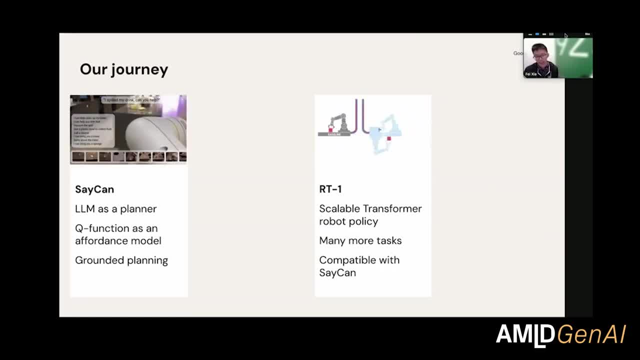 So then we developed RG1, which is a transparent robot policy that can manipulate things around the environment and pick up objects. It can do about 700 different tasks at a 97% success rate, So I've got a very Capable, loadable manipulation policy. 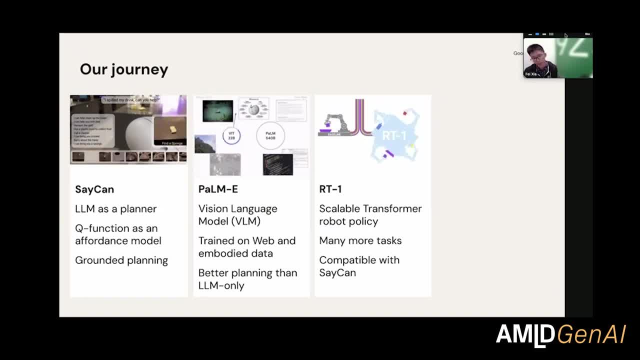 So after SayCAN we also did something on another model on a high level. It's called POM-E. It's the largest vision language model to date. It's a vision language model, So it takes in both image data and language data. 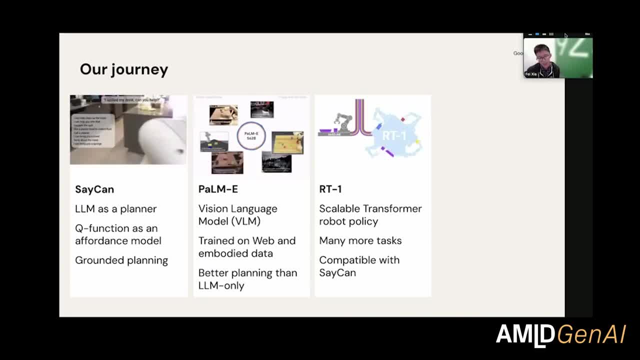 It's trained on both web and body data So it can do better planning than just using language models. So essentially, in SayCAN there's language model, There's value function, We provide them to do the planning. But in POM-E 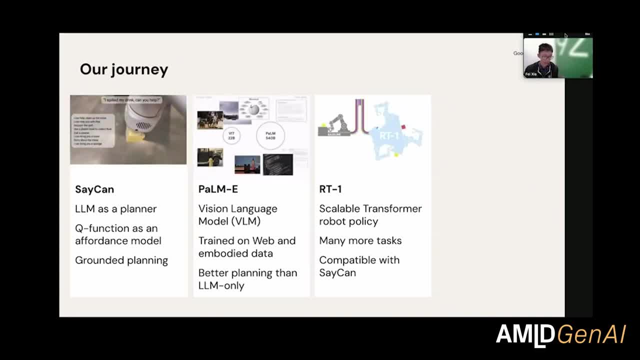 The value, function or the affordances are absorbed into the language model itself. So you can tell if a certain robot embodiment, it can plan with that certain robot embodiment in mind. And also recently we have RG2, which is a natural progression of RG1.. 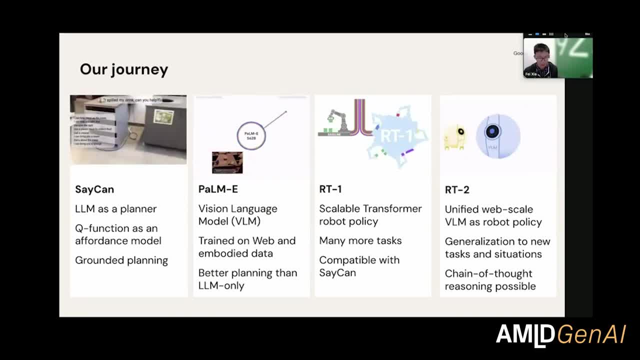 So RG1 is our first iteration of a robot transformer. RG2, we essentially unified the web scale BLM as a robot policy And it can generalize. It can generalize to new tasks and situations. You can even do something that is only possible. 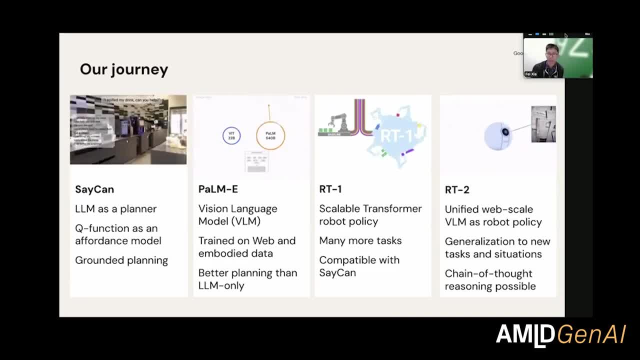 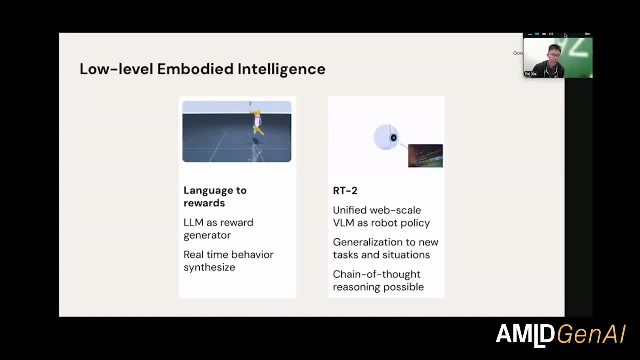 with a large-band model such as reason So you can do reason for robot manipulation. So in this talk I will focus on RG2 and another work I will talk about low-level intelligent intelligence. Essentially, how do we get to make a dog-like AI? 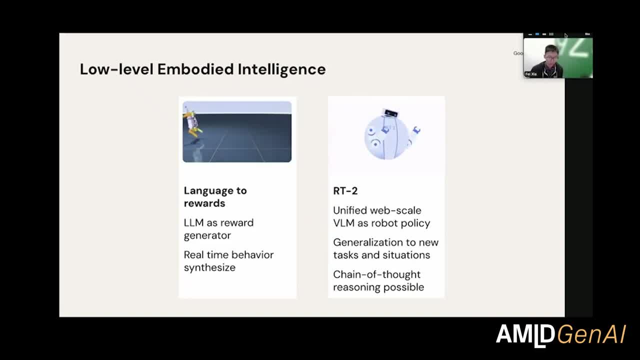 And I happen to have a dog here. So one work that I want to mention is language to rewards. So we use language model to generate reward functions and then do real-time behavior synthesis And then I'll talk about RG2.. We are still using formation models. 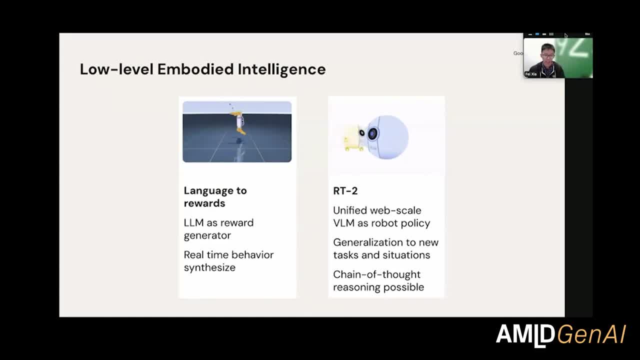 We're still using large language models. However, the problems of low-level embodied intelligence is much harder because you could argue that for a high-level reasoning or high-level embodied intelligence, it's closer to the large language model. So the large language model: it has to read a lot of books. 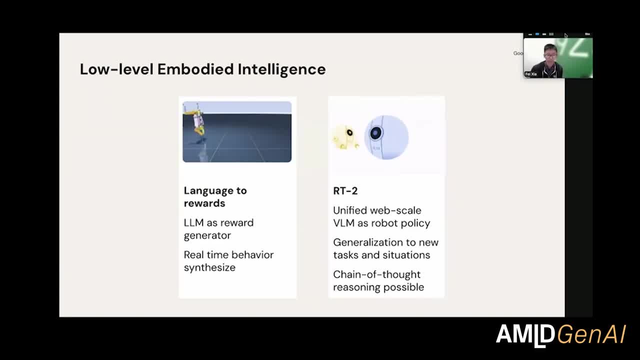 It has to read a lot of graphs, It has to read a lot of recipes And it happens to read all your wiki articles, So it has all this knowledge about planning and doing a certain task. However, it's much harder for language model. 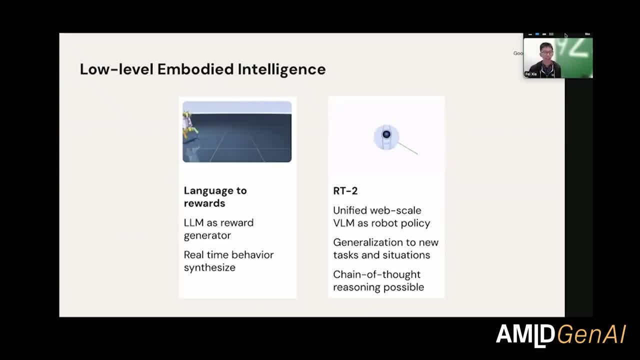 to reason that you need to move your hand to the right one centimeter, or you need to twist your arm, or you need to move your finger in a certain way. Those low-level motions are a lot harder, but it's not impossible. 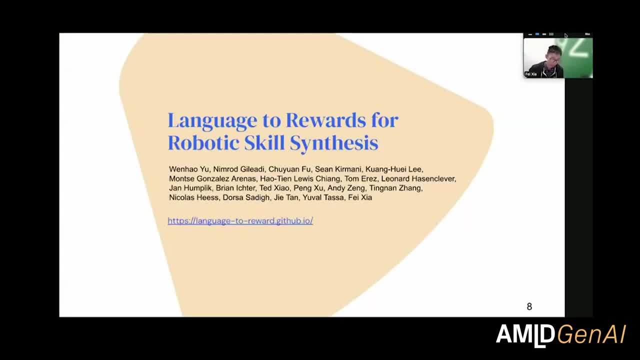 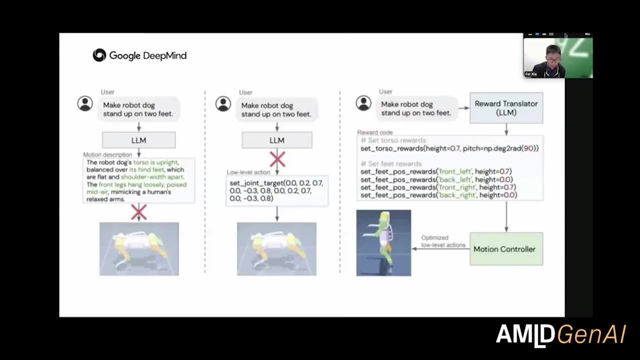 So there are two ways to do it. The first one I will talk about is language-to-rewards or robotic-scale synthesis, And it is a recent work with a lot of collaborators. The leading author is William Howe, and there was a Google big one. 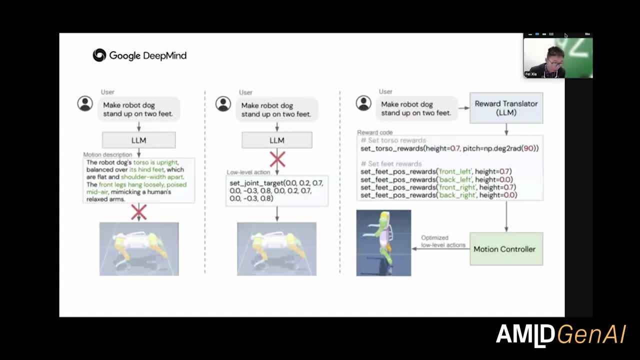 So let's assume we have this problem. We have a robot dog, A robot dog has a lot of degree of freedom and we want the robot dog to stand up on two feet. So we can directly ask the language model: how do you make a robot dog stand up on two feet? 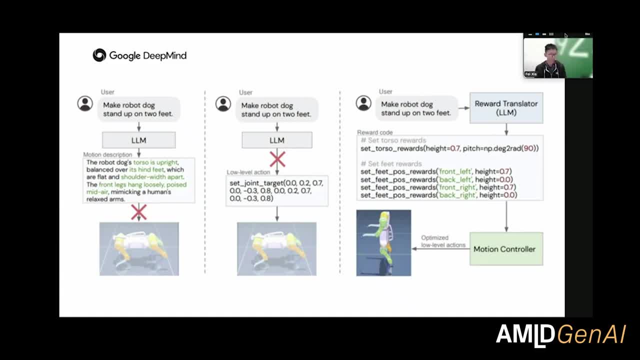 And it will recite a big parable back to you And upon reading it you find it's actually quite reasonable. So it says the robot also needs to be upright, It needs to balance on the high feet, And it also tells you something oddly specific. 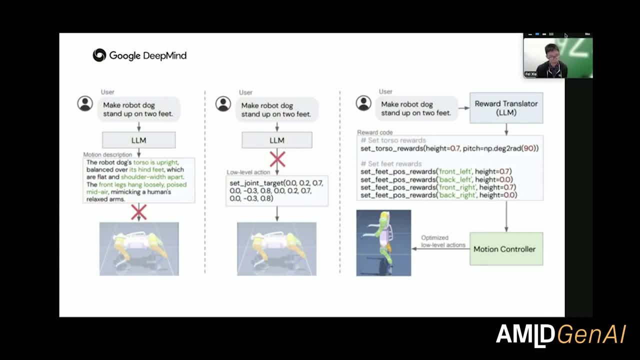 like the hand needs to be shoulder-width, apart from the leg to relax in the air. So these are all nuts, but the problem is that you cannot do anything about it. You cannot apply them on robots, So it's not clear how you translate those texts. 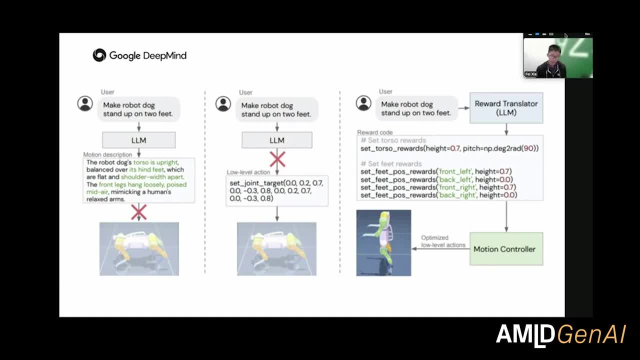 into robot motions. There is another way to do it. We have the robot API, So we obviously have a paper, but for this policy it's essentially using the program synthesis way of generating robot motions. However, here you will get kind of mixed results. 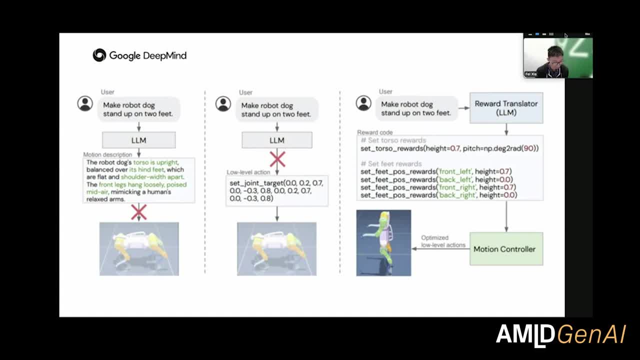 because the language model will not necessarily know your robot APIs and they don't know what the parameters means. So we propose a new framework. So we have a reward translator which translates the human instruction into a set of rewards. This is also a new way of viewing skills. 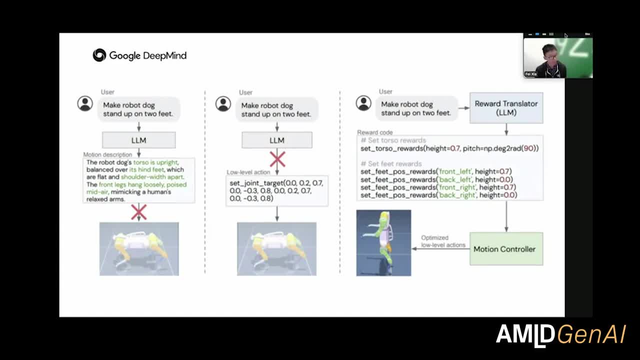 So one way to view skills is: it is a policy pie that maps observation to actions. Alternatively, you can also have a more higher level definition of skills. So the skills is a set of constraints and a set of objective functions. So take as an example: 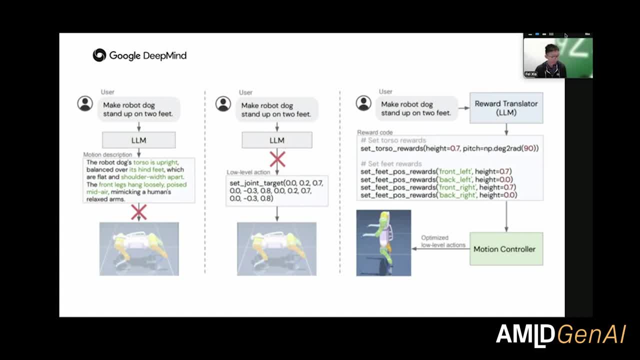 So picking up objects is a skill, But what it really means is your hand needs to be close to an object and the object needs to be off the so-called surface. This is arguably more generalizable representation of a skill, and they can be represented in reward. 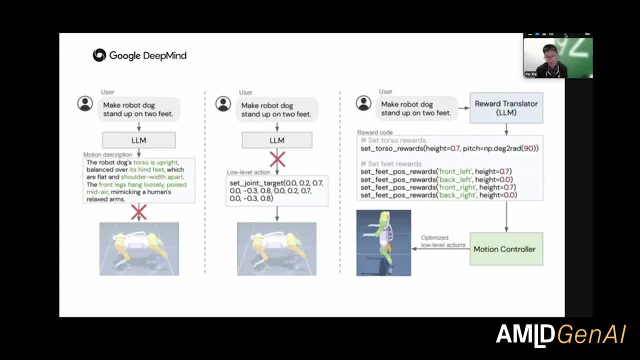 functions Other than the reward function. we can have a motion controller to generate the motion, So all you can use is reinforcement learning. So previously we haven't used reinforcement learning a lot, But in this particular work we use a black box optimizer. 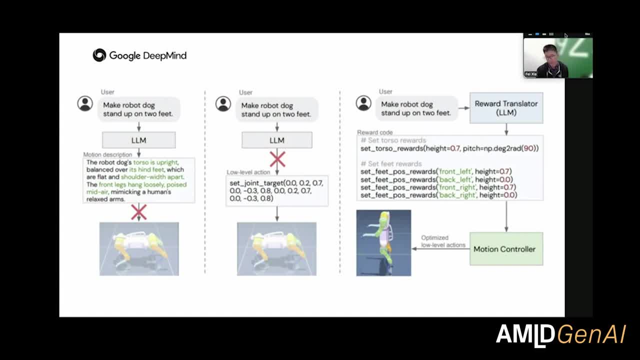 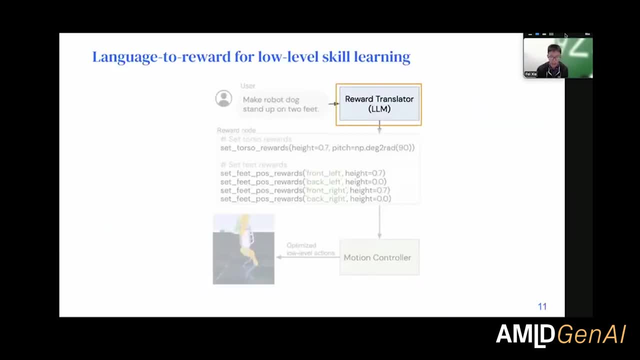 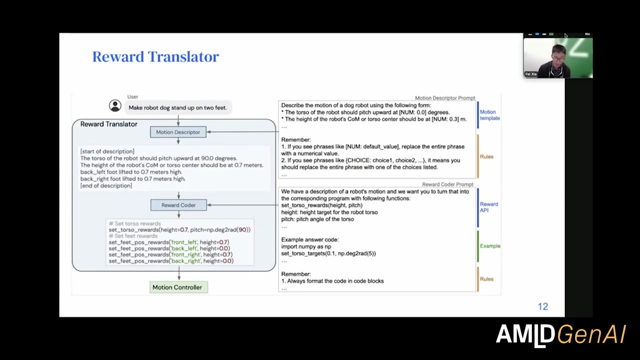 It's called Mojoco MTC, which can get motion in real time. So here is an illustration. Let's open the box for reward translator. So reward translator essentially is taking in the human instruction and then we're supposed to translate it to a description of the motion. 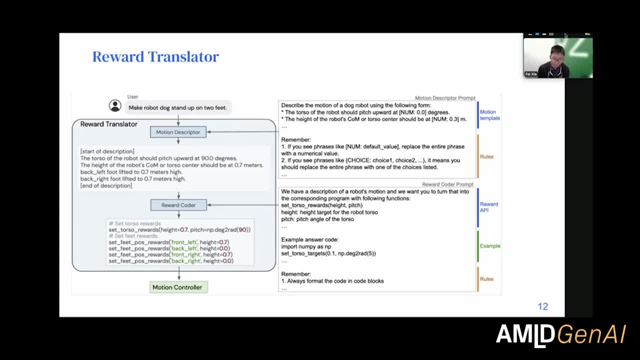 Remember, we see the description of motion and we quite like it, We think it's very useful. So we just ask the language model to describe this motion in a certain templated language, And then we have a reward: coder, which is a Python program synthesizer. 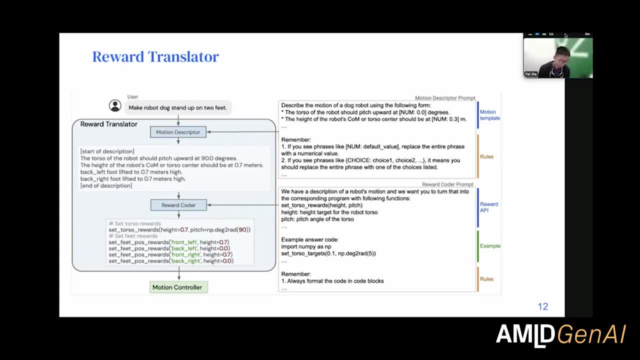 So both are just a language model with different prompts. We find this QState processor actually helpful because they can better extract the internet knowledge or knowledge about motions and apply them onto robots. The insight is that from the internet knowledge and purely robot motion, there is a huge domain gap. 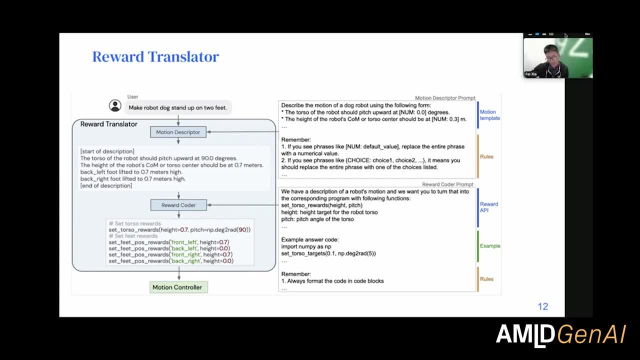 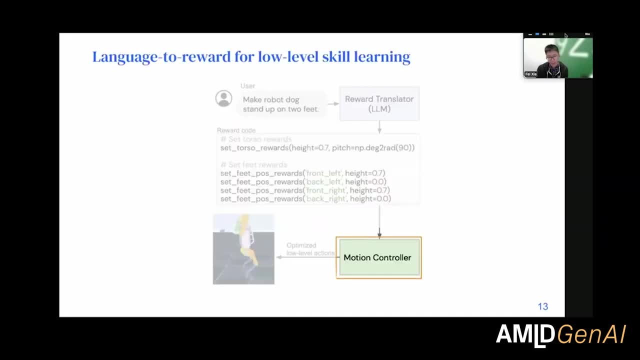 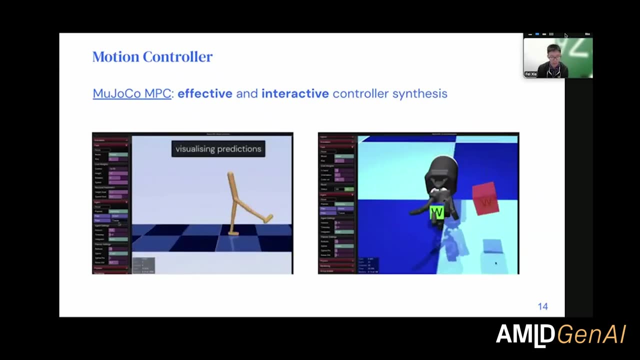 So you want to bridge this domain gap by going through some intermediate representations, And the motion description seems to be a go on. Let's take a look at the motion controller. So the motion controller is Mojoco MTC, which essentially is a black box optimizer. 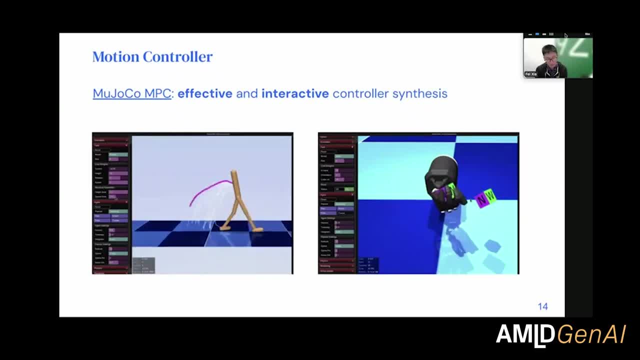 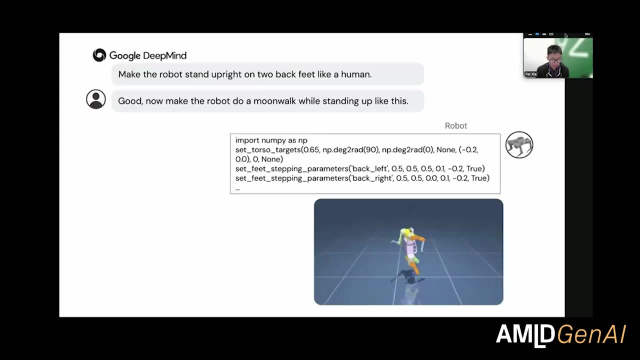 You can plug in any other black box optimizer here, But since we are using the simulated environment, it seems convenient to use this Mojoco MTC And it's really fast And it can generate a lot of different motions. So let's take a look at how this system works. 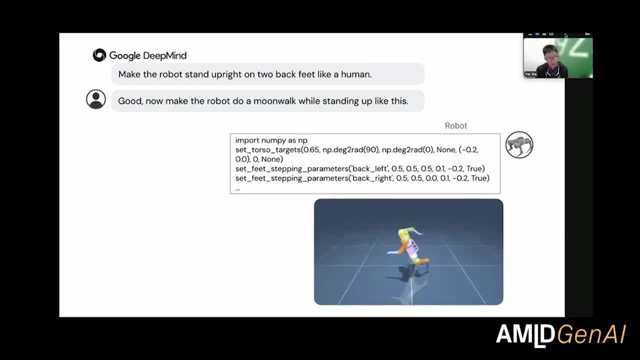 to give everyone a sense. So we can say: make the robot stand up on TV like a human, And it does that. Now we can even give it more requests because we're using language models. Language model is also a great user interface. 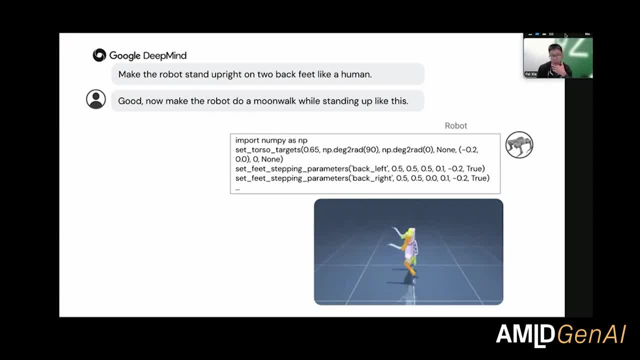 So you can give it additional instructions, You can give it corrections And they can say: OK, now make the robot do a little moonwalk while standing up like this. So we're getting a little bit more ambitious. We are trying to make it do the moonwalk in Michael Jackson style. 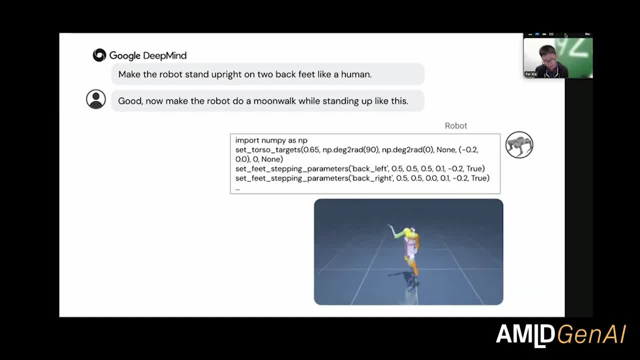 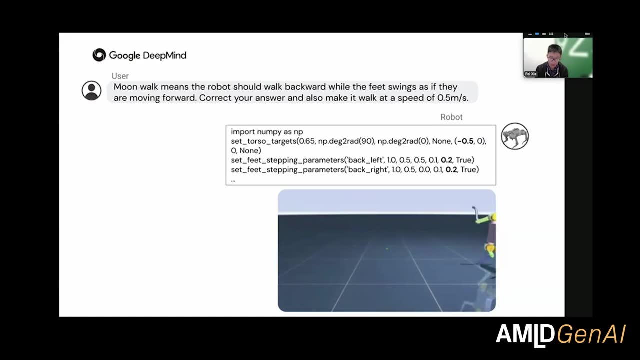 So the robot attempted something here. It generated a reward function and generated a motion. However, the motion is not exactly elegant. It's not the moonwalk that we are after. So then we can explain nicely to the robots that moonwalk means the robot should go backwards. 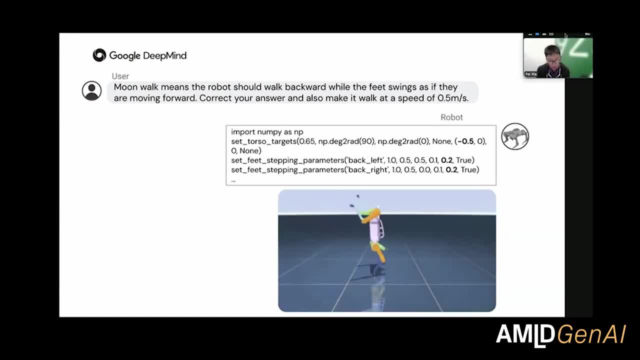 But the feet swings as if they are moving forward. Correct your answer And also make it walk at a speed of 0.5 meters per second And, as you can see, the language model surgically edits the code so that now we're. 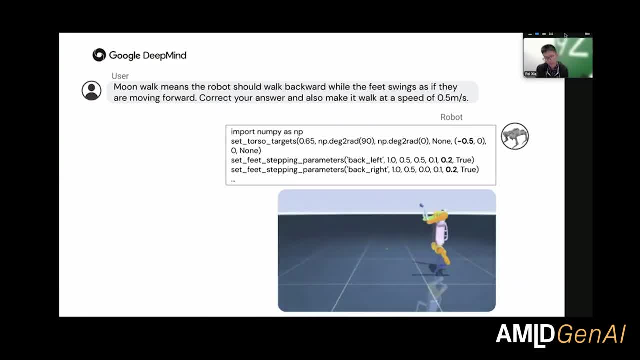 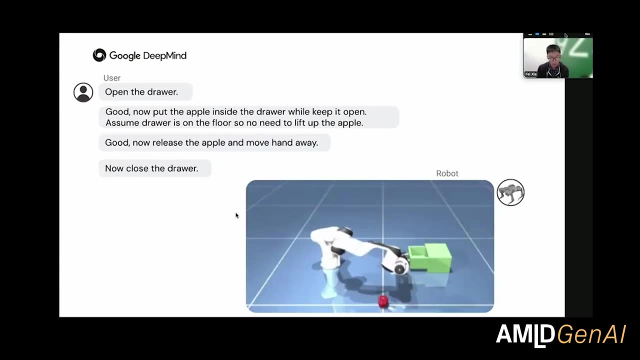 in a generator motion of the moonwalk. I'm not sure how the chips will show up through Zoom, But if not, you can go to language2rewardsgithubio to see this particular example And a ton of other examples. You can also teach a language model to do a procedure. 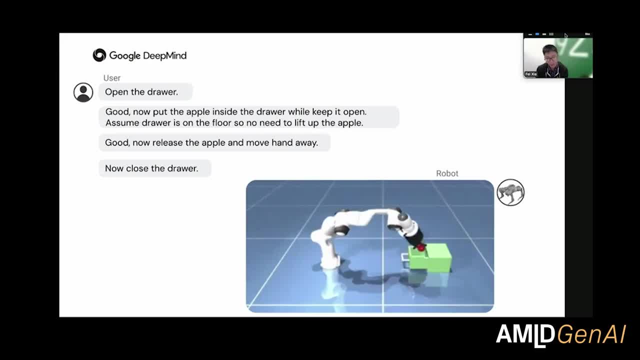 Like you can say, open the door, Put the apple in the door, Release the apple with the hand away and close the door. So this is a very high degree of freedom of the problem. So we mounted a shadow branta, A shadow or a shadow hand onto the branta arm. 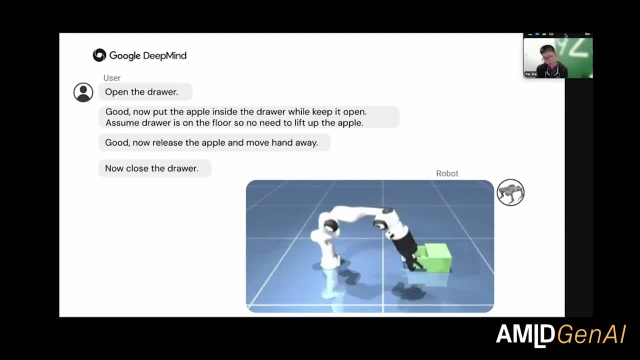 We call it shadow branta. It's a very high degree of freedom of control problem. But with the language2rewards you can go to language2rewardsgithubio to take a look. I guess I will take questions at the end. 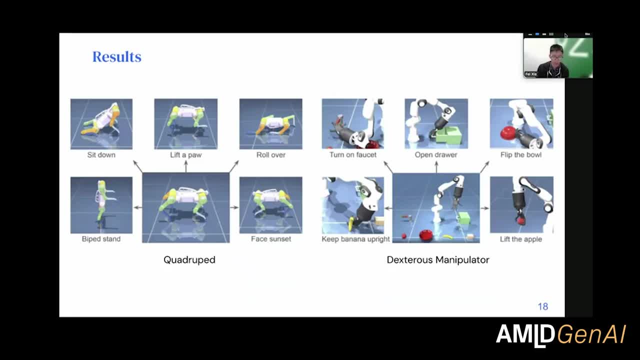 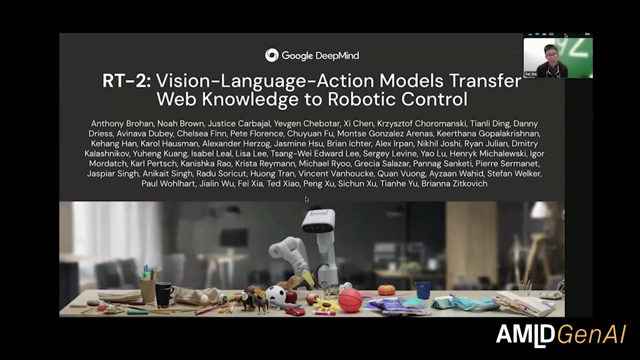 So I will move on to the second part of this talk, which is RT2.. So RT2 is our another attempt to create a new language model. So we're going to use RT2.. So we're going to use RT2.. So we're going to use RT2.. 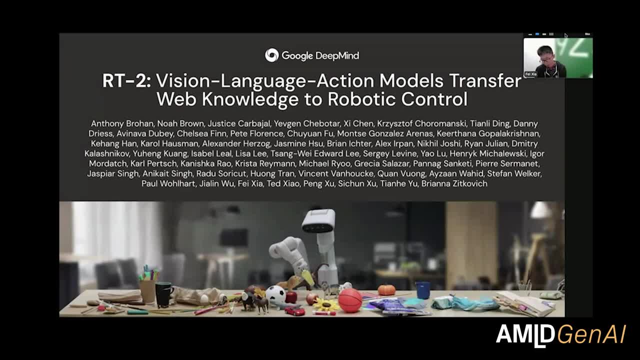 We're going to use RT2.. We're going to use RT2.. And this is our second attempt of using large language models to generate low-level motions. So we've already seen we can use the word function as a bias interface from the large language model. 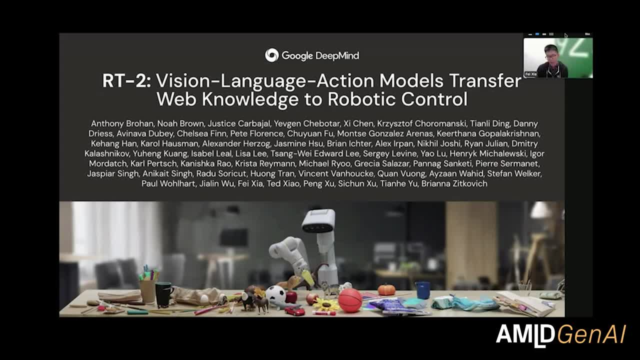 to generate low-level motions. So the RT2 is more like. can we generate the low-level motions directly from the language model? Can the language model speak global language? Can it directly output motor commands can fine-tune this visual language model so that they can also be a robot policy. 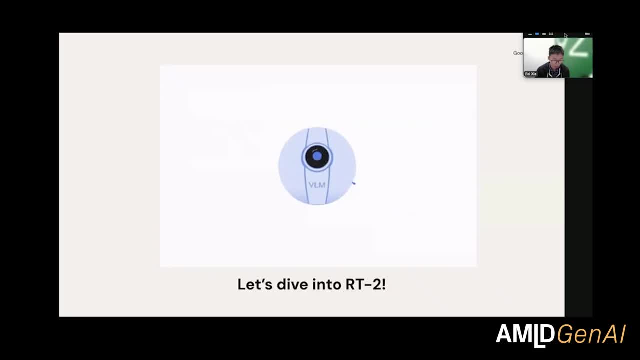 So the gist of RT2 is that we have a visual language model that is pre-trained on the internet data. So we have a big visual language model and then we can fine-tune it with only a little bit of robot data. So we use the RT1 data to fine-tune this visual language model and now Bellarmine can finish. 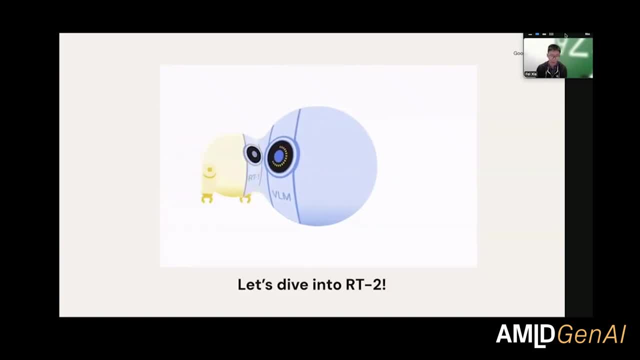 all the tasks in the RT1 training suite, but it can also generalize. it maintains some of the internet knowledge, some global knowledge inherited from the visual language model. So there is also a talk before this about visual pre-training. so essentially we are: 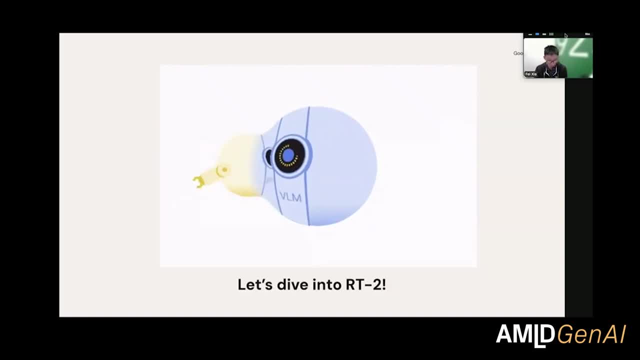 having the visual language pre-training in robotic policies. So it's just a visual language model, It's just a huge pipeline and curricula of tasks. So the brief introduction of the visual language model. I guess it doesn't require that much of an introduction. 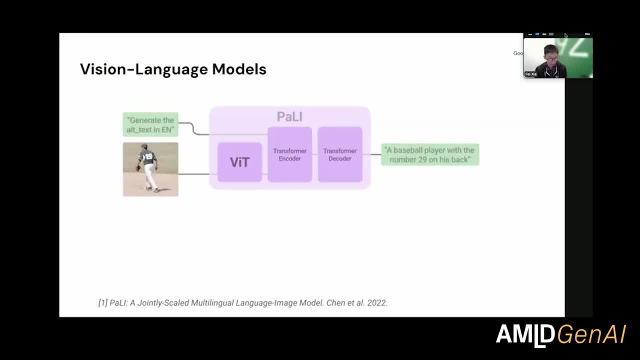 It's a model, a transformer model to be exact, and here is the encoder-de-coder model with a VIT visual path on top of it, and you can do a lot of different things with this visual language model. It's a very general representation of visual tasks. 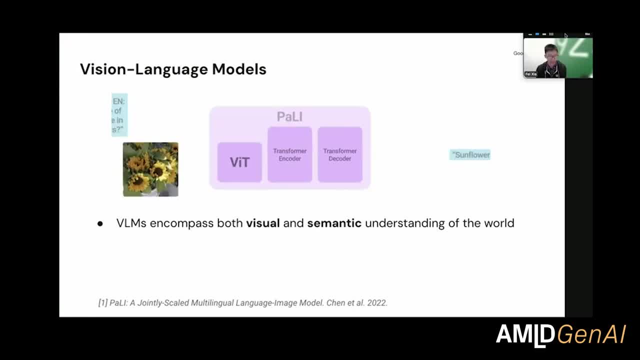 It's text and image in and then text out. The VLM encompasses both visual and semantic understanding of the world and you can ask it to do visual question answering and captioning and all other tasks, And those happen to be very important capabilities in robotics. 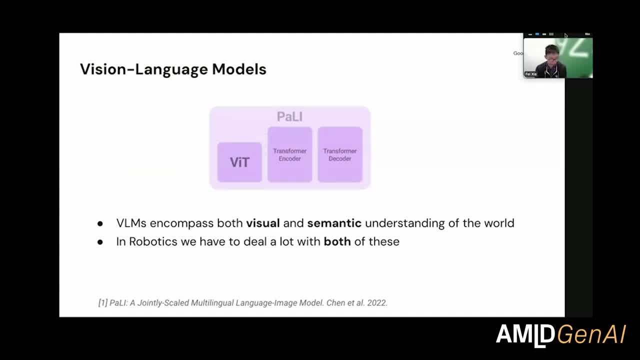 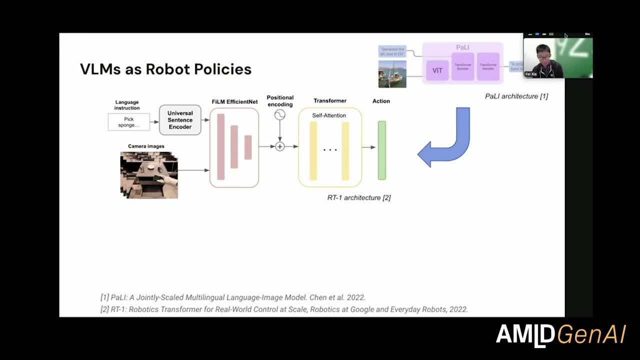 In robotics we have to deal with a lot of visual and semantic understanding, And now the question is: how do we leverage all of those knowledge? We can actually convert this visual language model into a robot policy. So here is a brief architecture showing the architecture of the RT-1.. 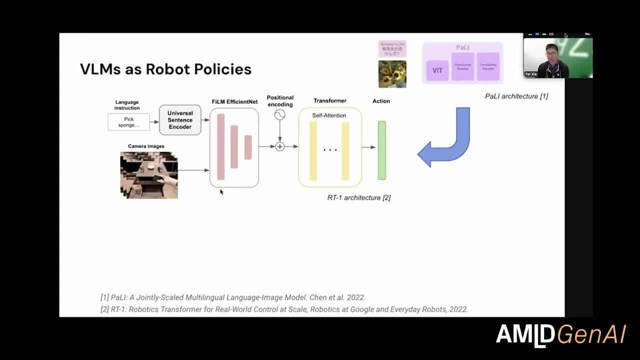 So RT-1 is also a robot policy, but it's not just any robot policy. It's a language-conditioned one, so it's conditioned on human instruction. So human-to-human instruction and a series of camera images. We have a transformer block, although a very efficient one. 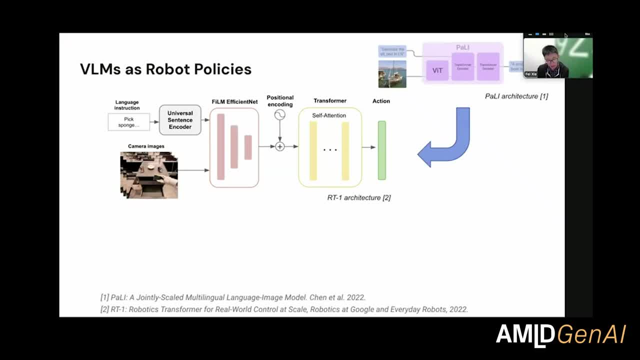 We developed some efficient transformer architecture so that we can run our robot in real time. We have it as a policy, We have this robotic transformer as a policy and it can generate actions. So we tokenize language, we tokenize camera images and we tokenize actions. 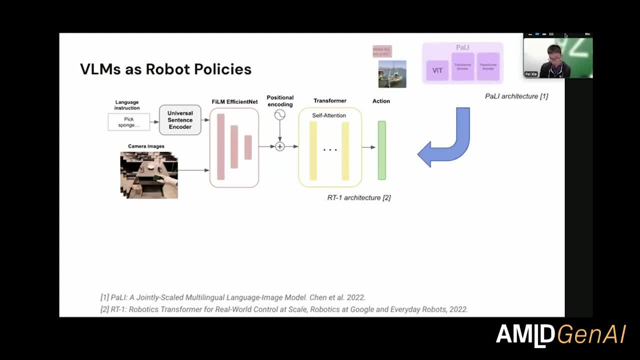 And then we can output those tokenized actions. So if we zoom out a little bit, the two architectures, the visual language model and the robot policy, are very, very similar. So RT-1 is also image plus text, plus two discrete robot actions. 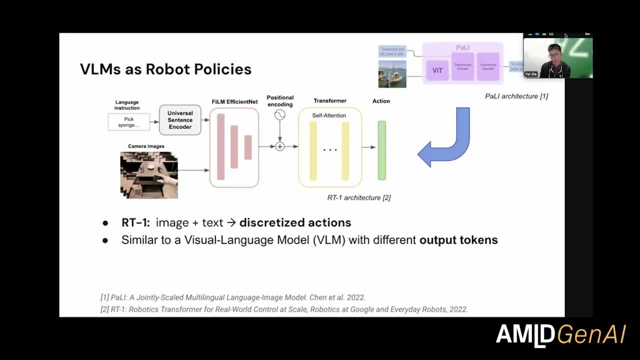 And it's quite similar to visual language models with different output tokens. The only thing is we need the visual language model to speak robot language, which are those action tokens. And we also have the question: if we do this type of monitoring, does this view maintain the robot language? 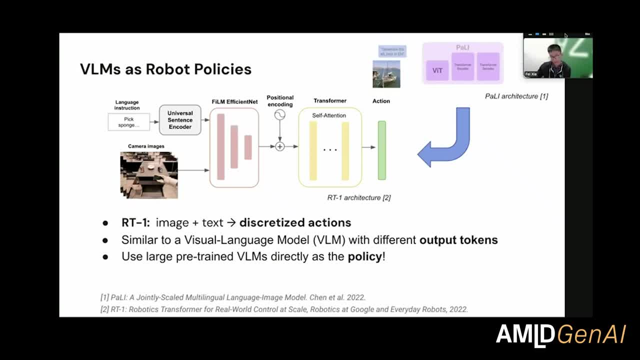 Does it maintain its visual understanding of the world Or it is essentially overfitted to the robot world? So that's something we want to figure out in RT-2.. So we can directly use the large between visual language models as a policy. 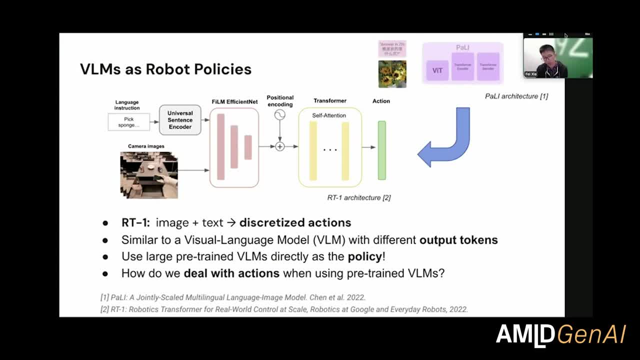 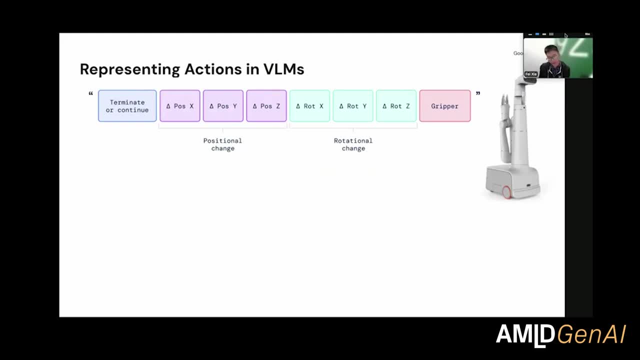 The other question is: how do we deal with actions when using the briefing VLMs? So here is how we represent actions in VLMs And I would like to say that this is the active research direction. So there are many different ways for you to deal with action representation. 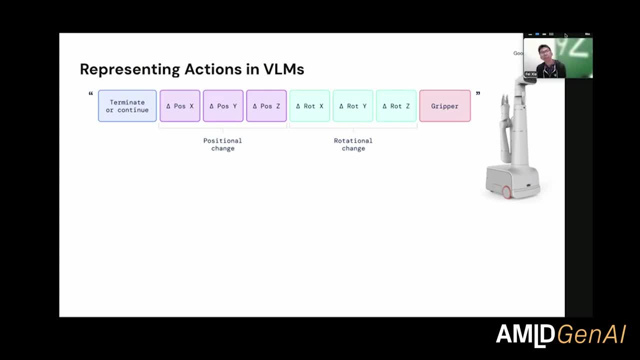 Some action representations happen to be more, let's say, efficient or slightly better sample efficiency or easy to learn, like how friendly it is to VLMs or how easy it is to transfer knowledge from visual language models to robot policies. 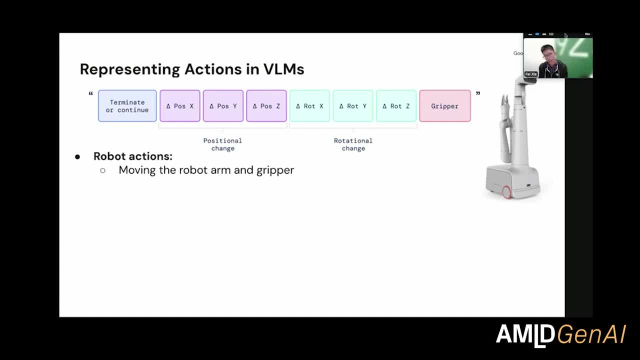 Different action representations are active. So our robots. it's also depending on the robot. Our robots can have 70 degree of freedom, arm with a gripper. So we represent everything using the anti-effector, essentially the gripper, delta pose and the gripper closeness. 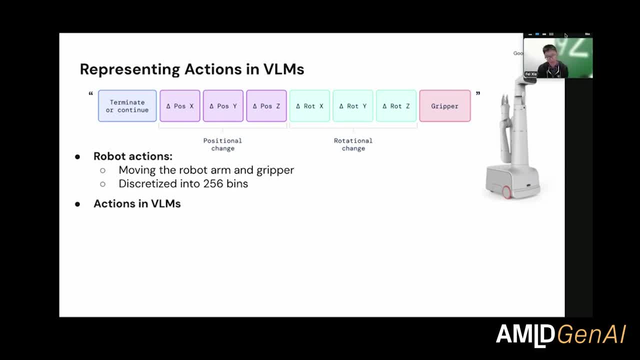 So there are eight dimensions of the actions. We discrete each into 256 bins and we convert it to a string of numbers. We're literally just using a string of numbers. It's probably not the most efficient representation, but we find it works. 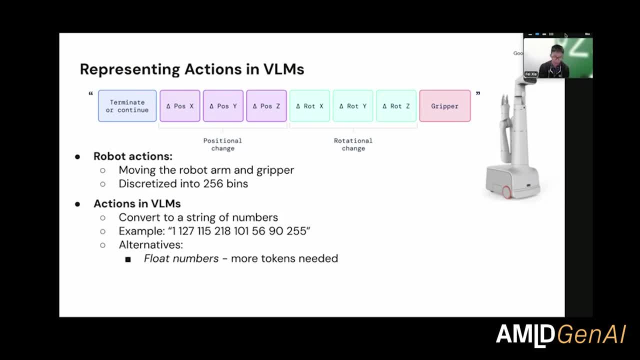 We tried some other things: Floating numbers. Floating numbers require small tokens. Language model is not the best at understanding decimals. We also convert it to human language, left or right, But it's also ambiguous. It cannot be directly executed on the robot. 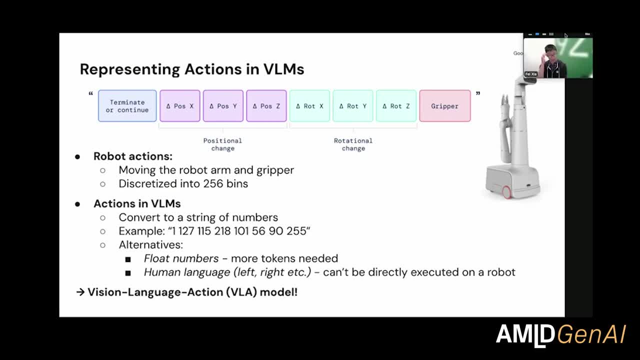 And we, after playing the robot action representation, we settled on this discrete naming of eight dimensions And we find it empirically to be working well, although we might be able to find better action representations. After this last piece, we now have a visual language action model. 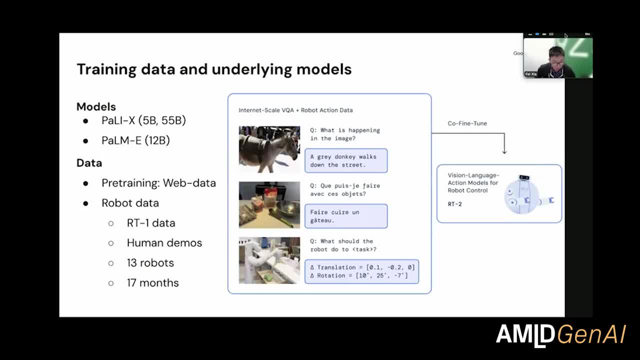 We have two architectures, One is and another one is. So the data to train these, to train the visual language model, is, of course, the web data, And after that we combine it with some robot data. We use the same RT1 data so we can have a better comparison with RT1.. 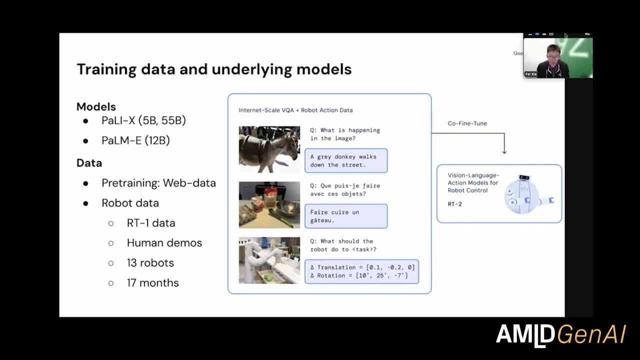 There are human demonstrations collected by physical robots over 70 miles, And then we have a procedure called co-fine-tuning. Essentially, we just add the robot data into the pertinent mix. We are not just fine-tuning on the robot data. 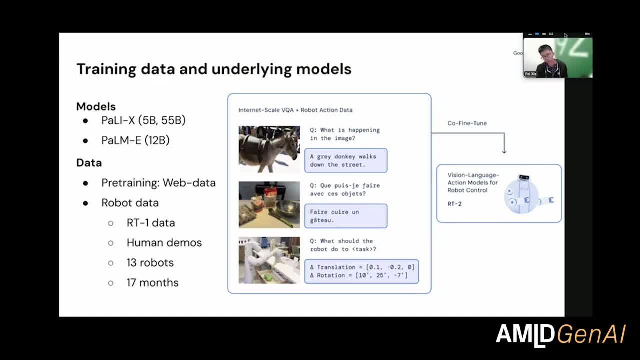 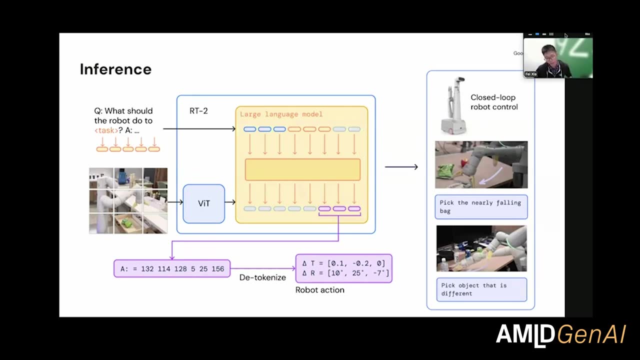 because we worry about overfitting- And it seems that the co-fine-tuning procedure also has some advantages of maintaining the visual language capability of this real animal- And, at inverse time, what we end up doing is we essentially use the BLM as a policy. 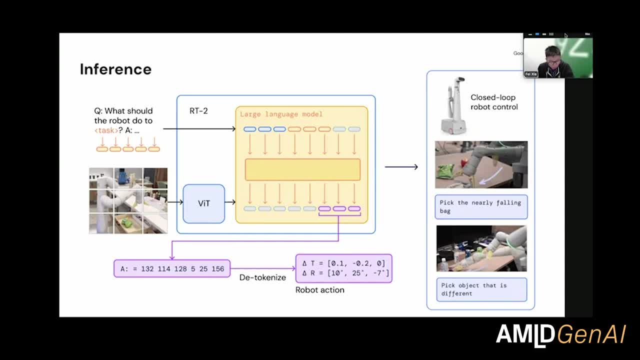 We can have a tokenized text and image input and we have the tokenized action output, which is eight numbers. Each of them is between 0 to 255. And we can depokenize them into developers and directly execute them on the robot. 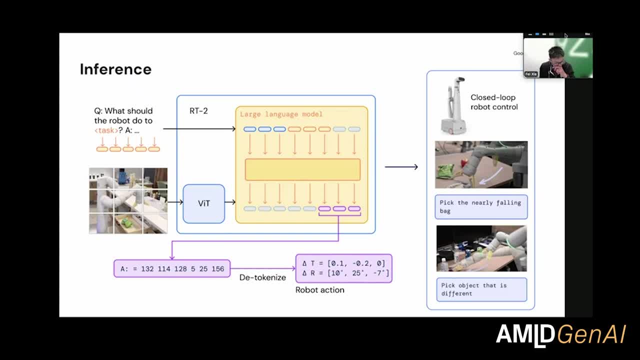 And we do this in a closed-loop manner. The visual language model can actually run pretty fast on the cloud, So we can run it up to three hertz. We can have this closed-loop control of getting the observation generating action and then essentially do this over and over again. 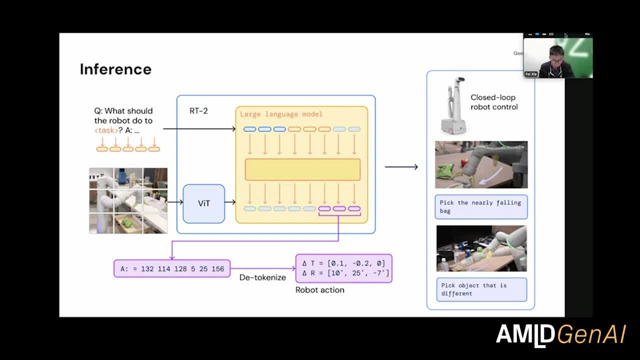 until it finishes some tasks. So we find we can do some quite interesting tasks, including pick the nearly falling bag, the reason about which bag is nearly falling, and pick out the object. that is different, But I'll go more into details in a little bit. 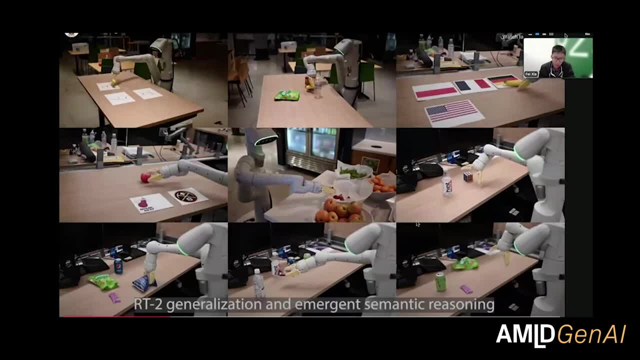 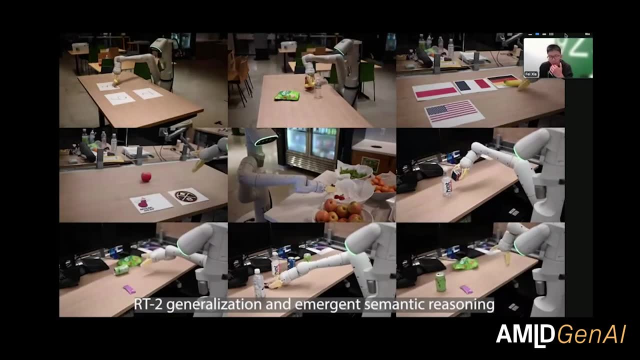 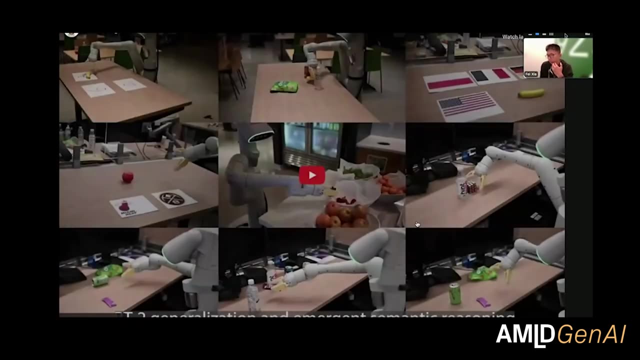 So here is an illustration of the tasks that they can do. So all of these tasks are out of distribution. They are not in the RT1 chain distribution. So we are playing with the policies the same way. the playlists try to be key. We essentially just prompt it with different things. 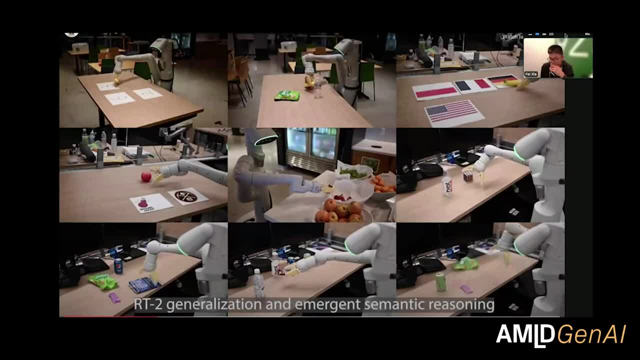 just like testing intelligence of a three-year-old, for example. The other thing is that a lot of the objects are the robots, like I have already seen it in the training data, So we literally need to run to the dollar store to buy a bunch of toys. 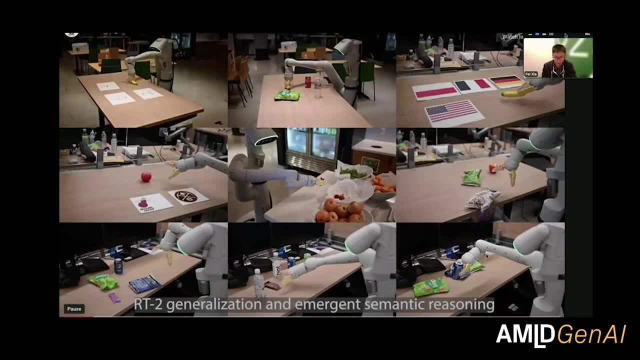 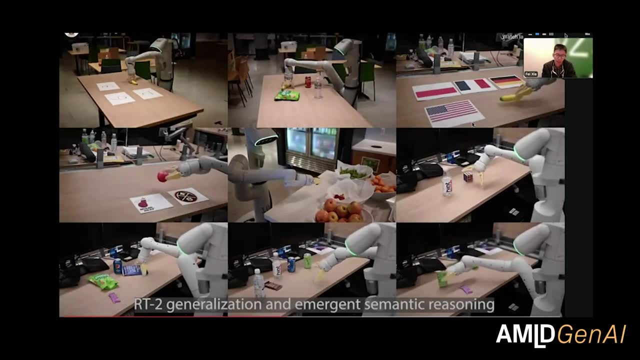 and then to test the generalization capability of the robots So it can do things like move the banana to German black on the top right. So it understands different blacks, It has a semantic understanding of different things. And in the middle just put the strawberry. 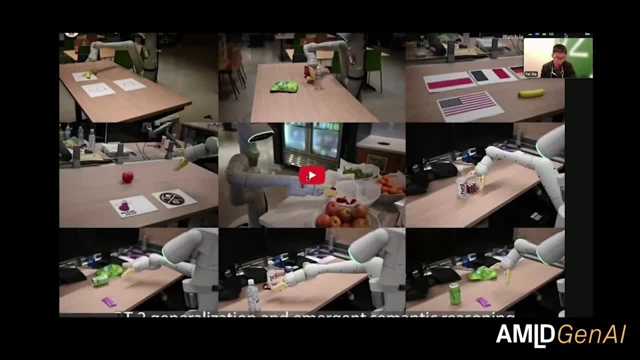 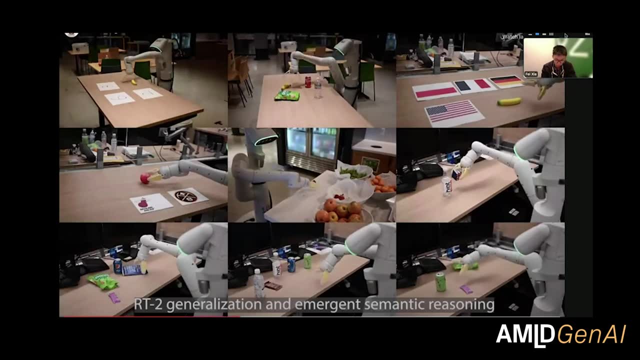 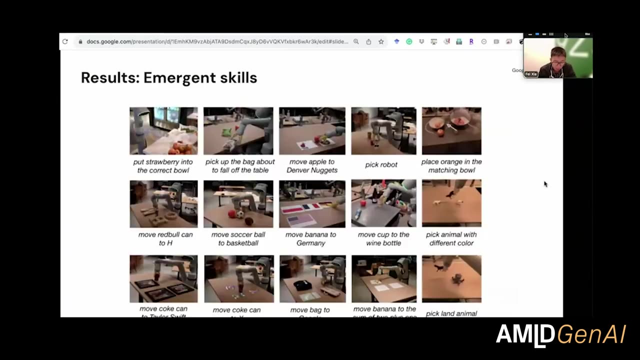 and grab the ball. So you need to understand what is the strawberry- Grab the ball means strawberry ball- And then do this sort of one-off reading and association. So I think these are pretty cool capabilities. Yes, so here are a list of tasks. 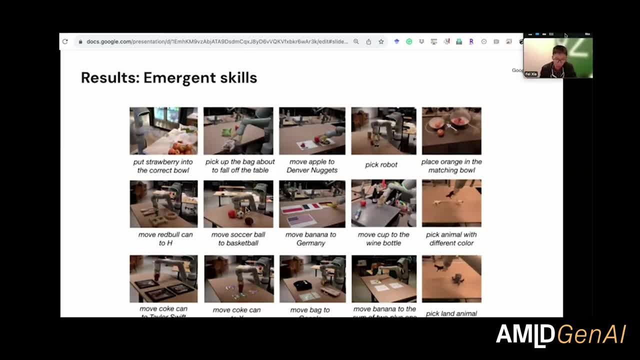 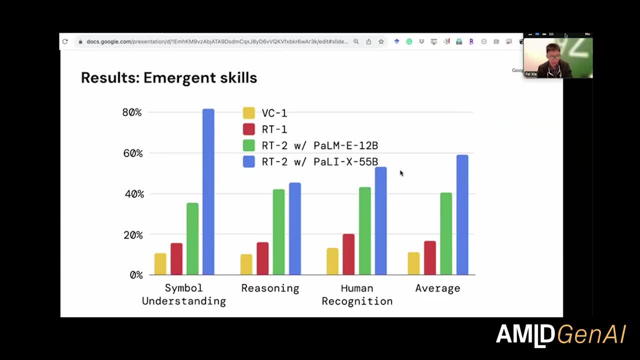 So for more details, please go into read our paper and we have more of the skills to show. We did some benchmarking Of how these compare with other robot models, including VC1, which is another ratio model control policy, And we compare with SCAR-1,. 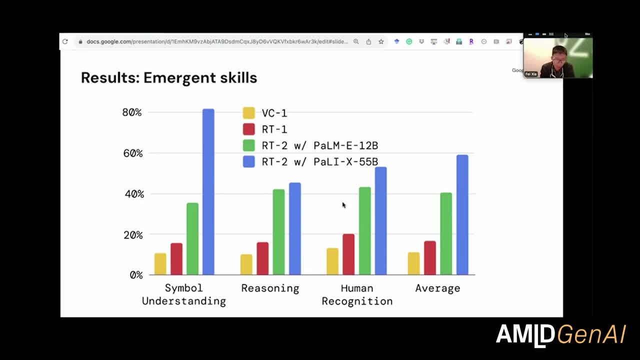 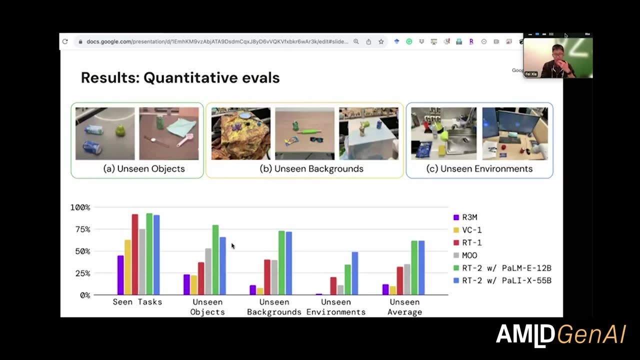 with iteration of robot transformer And we find that the IT2 performs much better in those tasks. that requires some code knowledge or requires semantic knowledge, Right, We also find it is more robust to, let's say, background noise, unseen background. It generalizes better in unseen environments. 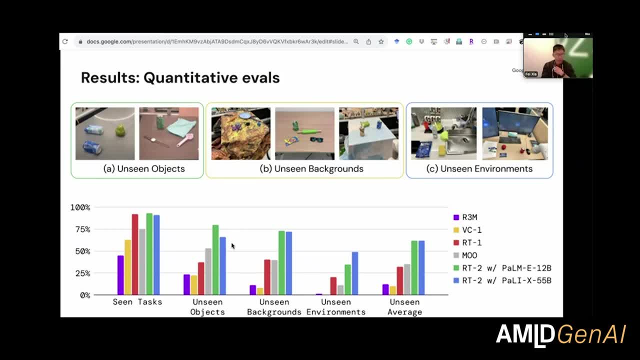 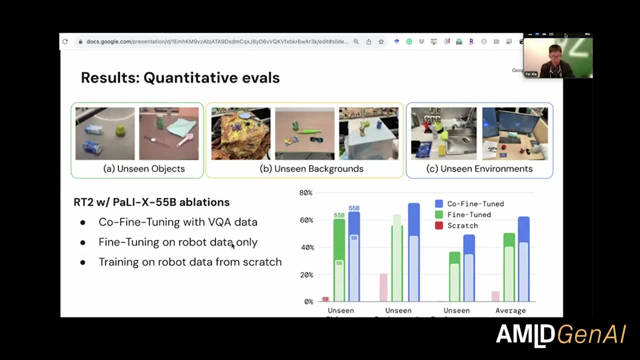 Right, So this should be the IT2.. I will then go to detail into the quantitative results, But we find co-fine tuning helps. Co-fine tuning helps you maintain the visual capability of these models And fine tuning on robot data you probably have better in-distribution performance. 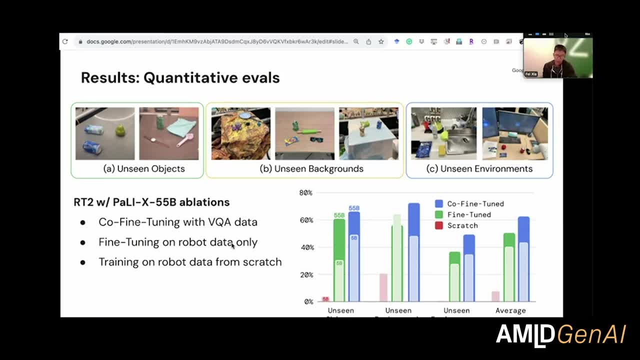 but then your auto-distribution performance is a little bit worse And training on robot data from scratch barely works. So you do need a large pre-training procedure of the visual language model before you can fine-tuning on the robot data. And maybe it's another signal that the robot data 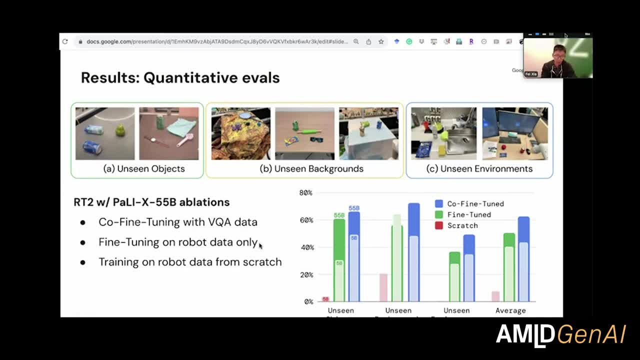 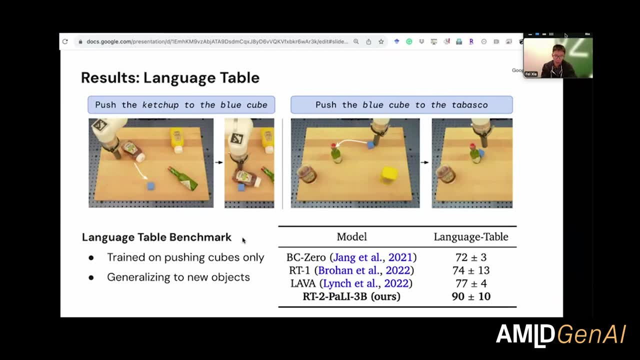 is just not enough to make the visual language model converge. We also tried another environment, So this is also. we can use the same model in different environments And it can essentially calibrate averages and distributions of each environment And it can do different tasks. 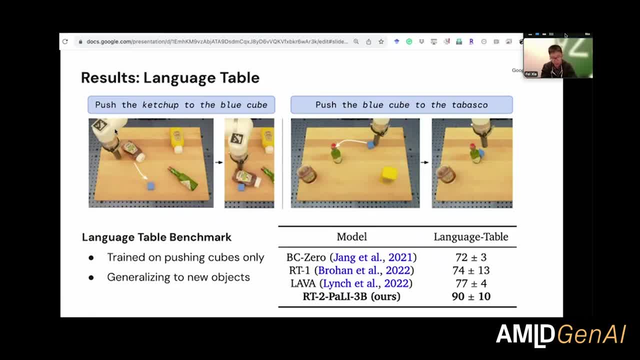 So this is a tabletop environment. It can also ask you to push the catch-up to the blue cube, So the catch-up is actually auto-distribution. It has never seen catch-up before. But well, it has never seen catch-up before. 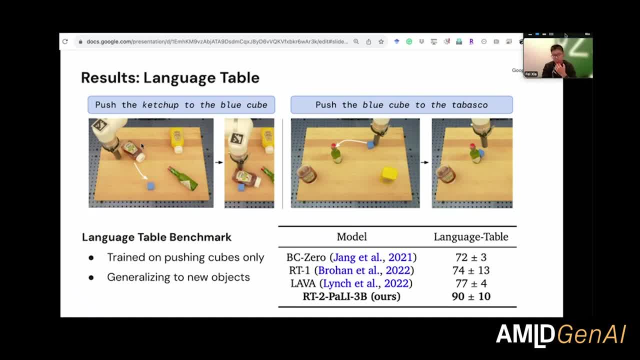 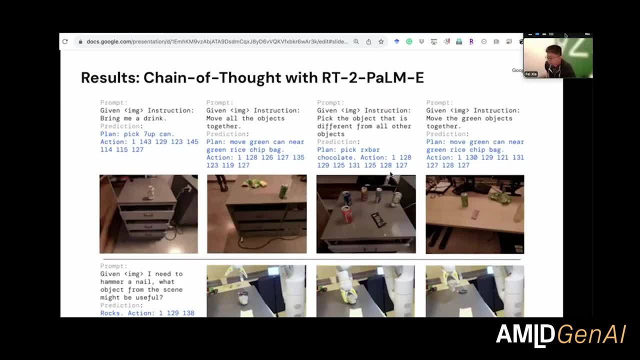 in the robot training data, I should say, But it's able to do this task And it was high signal rate. One interesting thing is the reason. So reasoning is a prompting method in the, which was proposed by Jason and a few of my other colleagues. 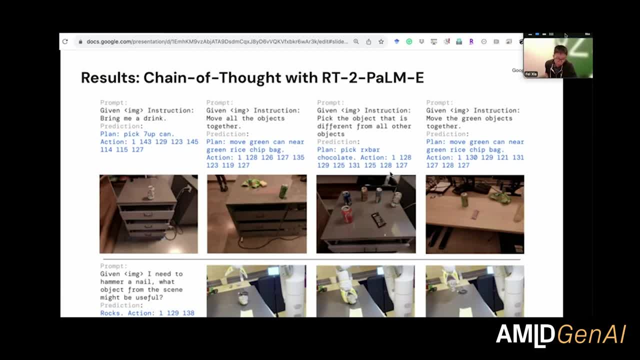 So we can tell about reasoning with a visual language model too, and also a robot. It's a very interesting experiment. So essentially the way to do it is: we have this pre-trained RGT model and we fine-tune a little bit of data. 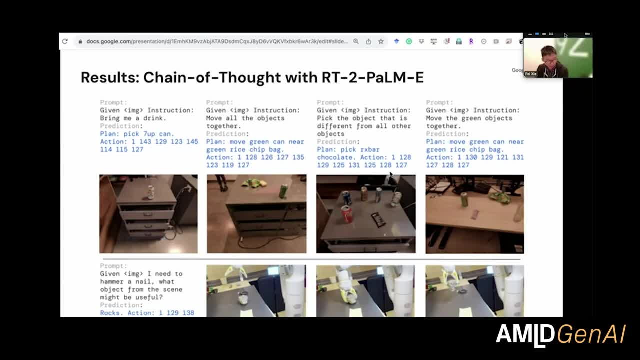 maybe a couple of hundreds of data. that contains a prompt, a plan and an action, So it has an intermediate class. It's not completely in-context learning So it requires a little bit of training But it doesn't require a ton of data. 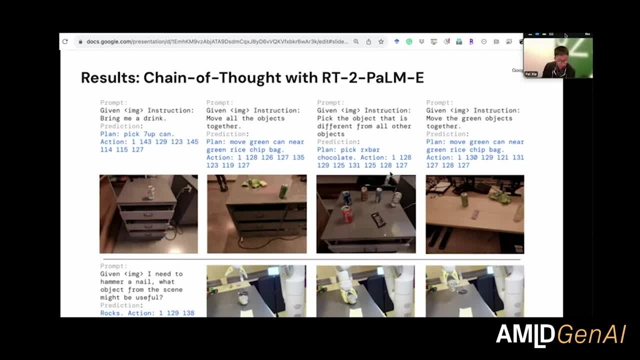 It's more like calibrating the optimal format to a different new format, And with this chain of thought reasoning you can make it: generate a plan and then generate actions. And you can do more complicated tasks just with generating data and then generate actions. 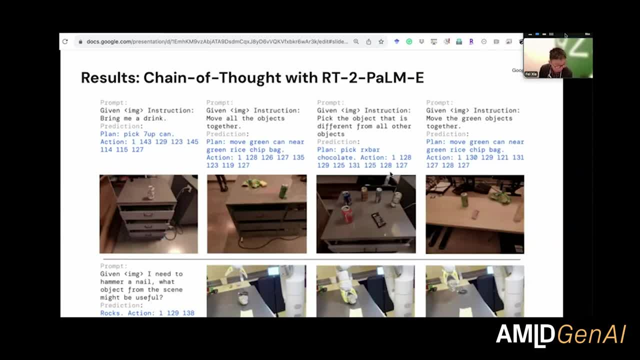 So one interesting experiment we did is to put on the table a rock, a piece of paper and a headset, And then we asked the given image to hammer a nail where the object on the scene might be useful- And it says rock- And then generate actions to pick up the rock. 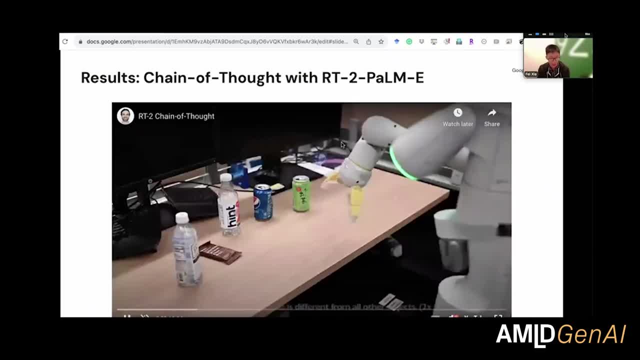 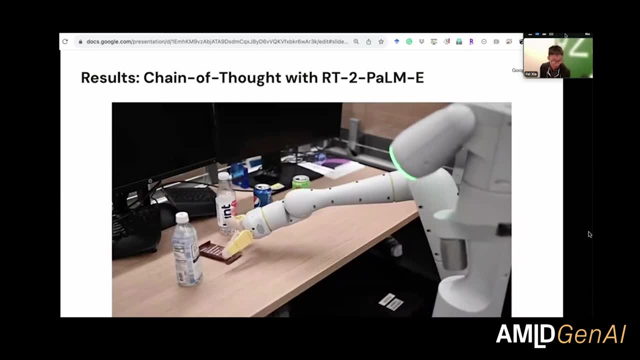 So this is just one example where you can do a lot of different things because we have that model. So another thing that we did is to ask you to pick up the object that is different. What does different mean? Different means: well, this is a snack. 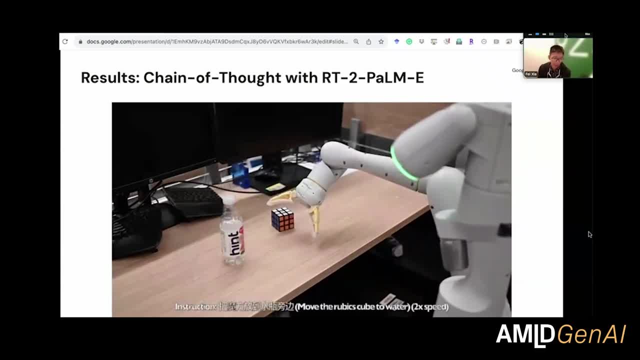 The rest of the objects are things You have to pick up the snack. You can also ask things in other languages, And the plan would essentially be to translate this into English, So it gives you more opportunity to bridge the gap between different domains. 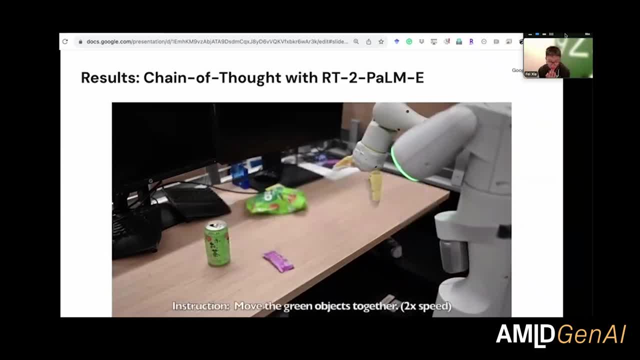 So the last example that I want to show is to move the brain objects together. So this is actually kind of interesting, because the plan actually oscillated a little bit. So you can move brain object one to brain object two, But you can also move brain object two. 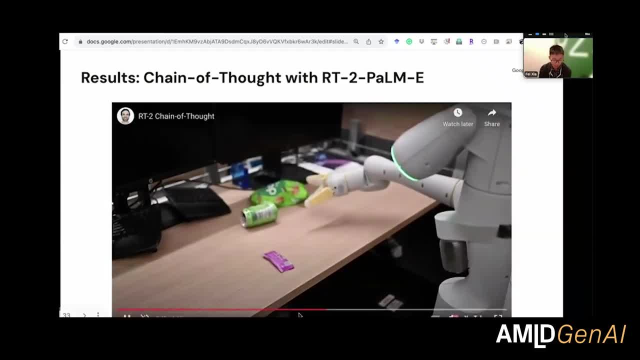 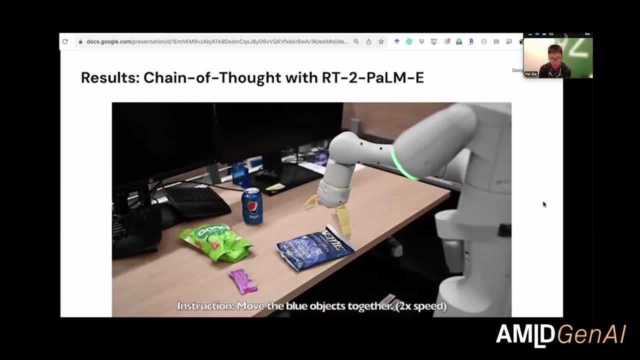 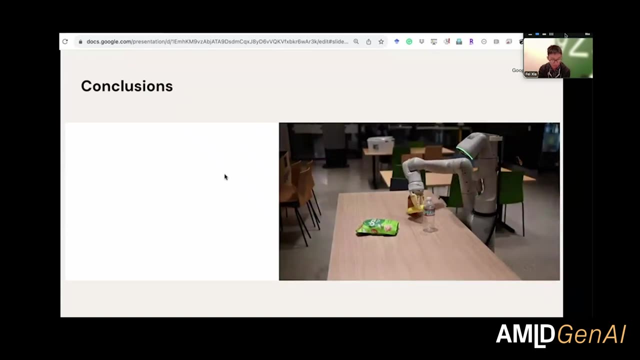 to brain object one, And it oscillated a little bit. And then, once it's closed, once it's closed enough to one object, then it's committed to the object and finishes the task. All right. So, finally, I would like to conclude this talk. 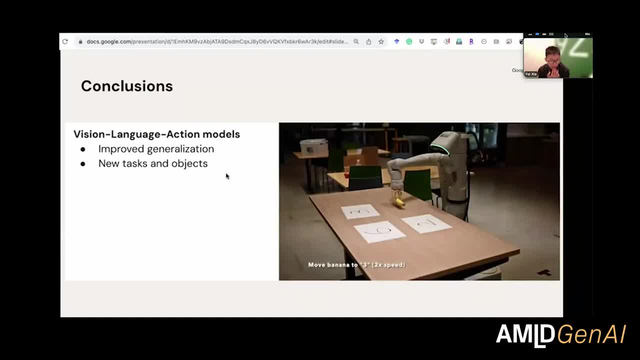 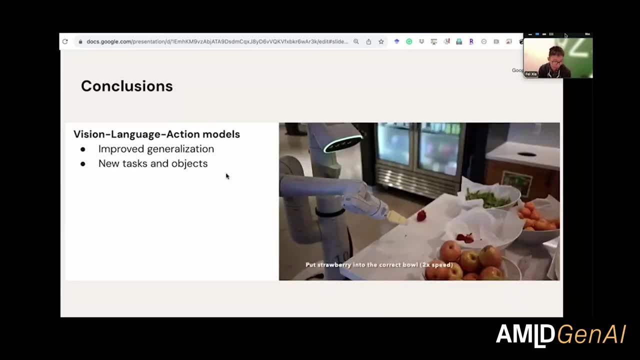 So we have a visual management model that can improve generalization. We have this RGT model. It can work on green tasks and new objects. It can even do quantified reasoning And it includes the underlying model, Including the underlying visual management model. 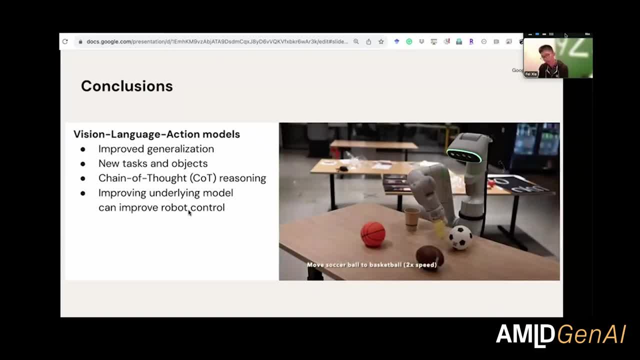 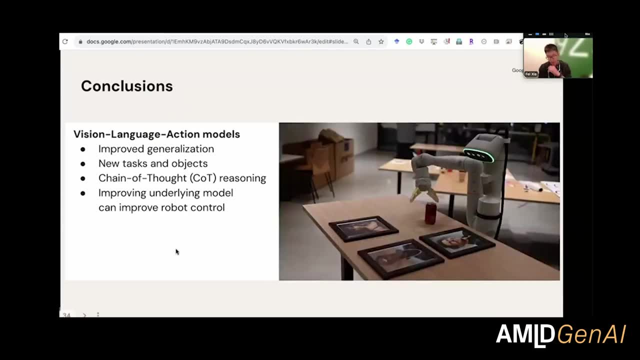 can improve robot control. So we see a lot of transfer from a visual management model to robots And it can be a lot of novel tasks. So essentially we've used the visual management model and the robot policy in the program and we see a lot of generalization. 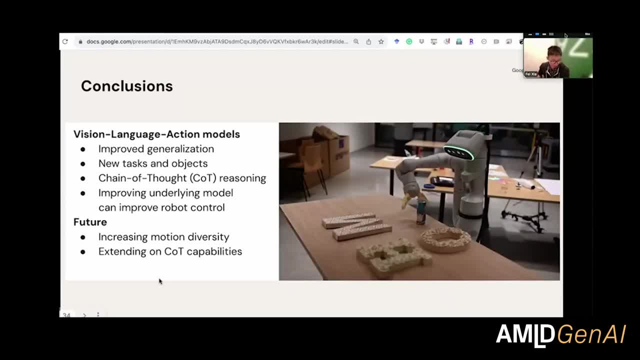 In the future. we want to increase the monitoring diversity, So we currently require protein visual management model or robot data to end up resulting in a very highly recognized robot policy. So it maybe doesn't have the motion diversity that we want. We also want to extend. 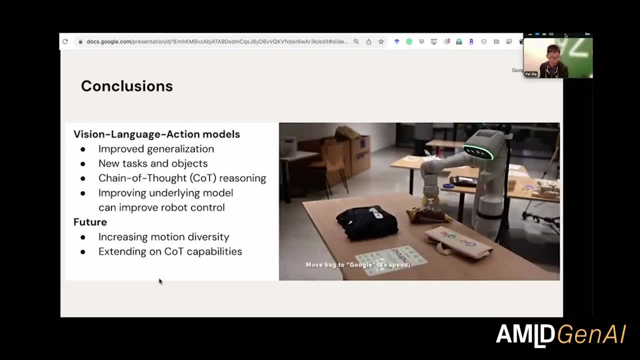 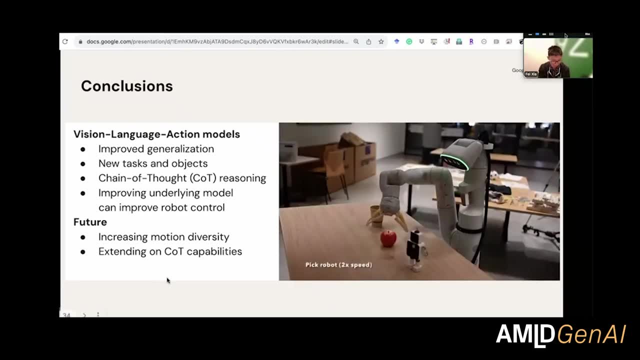 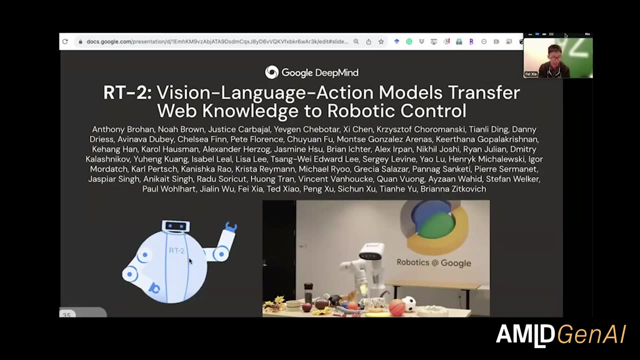 the chain of thought capabilities to more planning, more complicated planning and reading tasks, And then we want the director to explore this problem. So this is again a collaboration with many colleagues in our team and it's a huge amount of work, So kudos to folks. 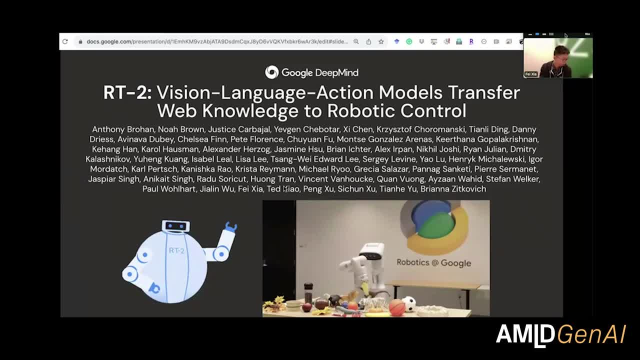 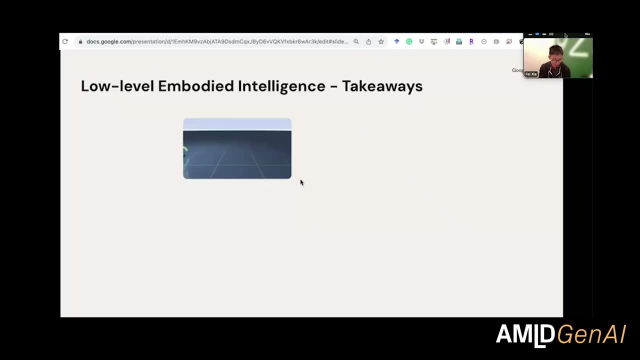 who made this work possible. Kudos to other teams, like Neil also did a talk earlier today. So the mission platformer is also a key component and the visual language model is a key component in our line of work. So to conclude my talk, 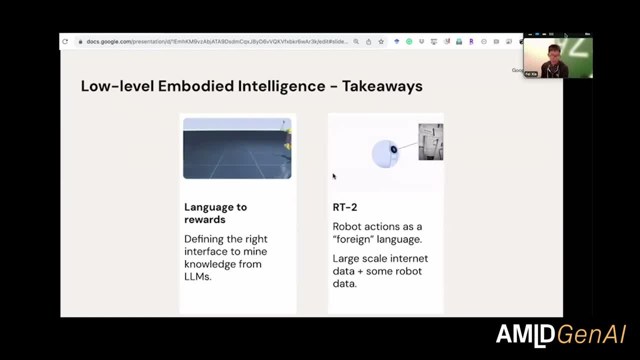 we made some progress in getting a lot of robotic intelligence. We can. we need to define a viable base to mine our robotic intelligence models and we worked on this in 1991.. And also, we can treat robot action as a foreign language, The moment we treat 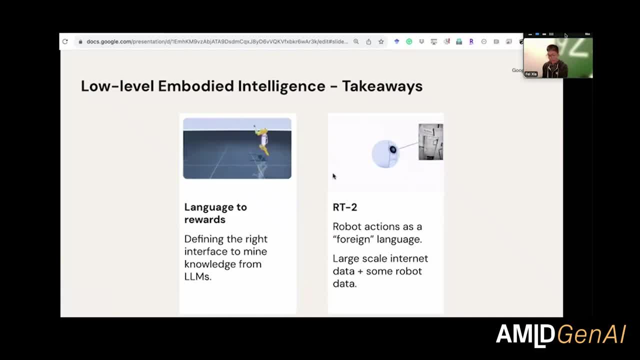 robot action as a foreign language. we can borrow some knowledge from the protein mix and then apply them onto the bodies And then we can do large-scale independent data plus some robot data. that enables generalization and more robust robot policies. Thank you so much. 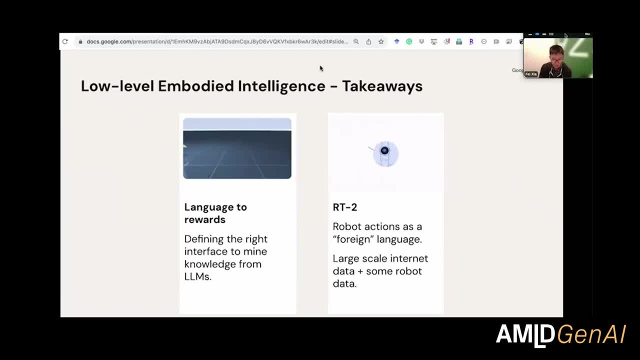 Let me know if you have any questions. Questions, okay, Hello. Thank you very much for the talk. It's very interesting. I'd like to ask: from what I understand like the robot policies are explicitly fighting the detaining data. 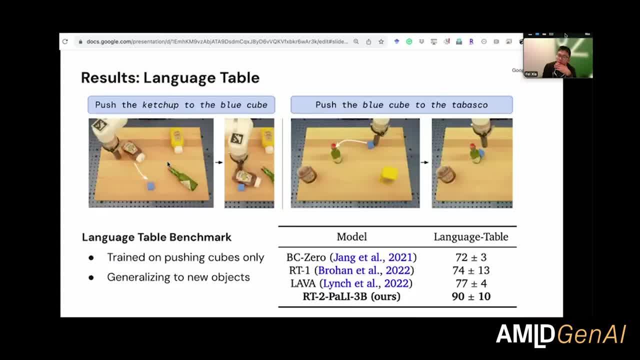 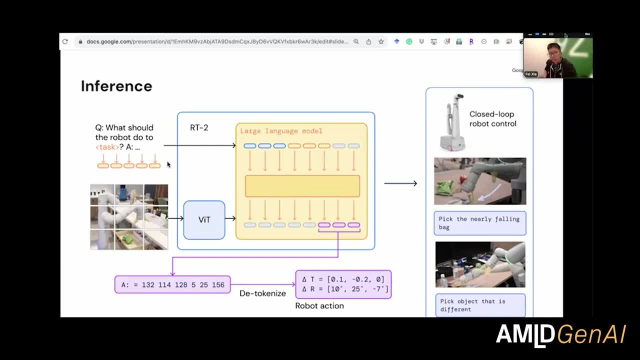 So do you think there is a way to combine this with reinforcement learning and to make the robot explore the actions on its own? Yeah, I think that's a super good question. So currently we are using behavior polling, We are using human demonstration. 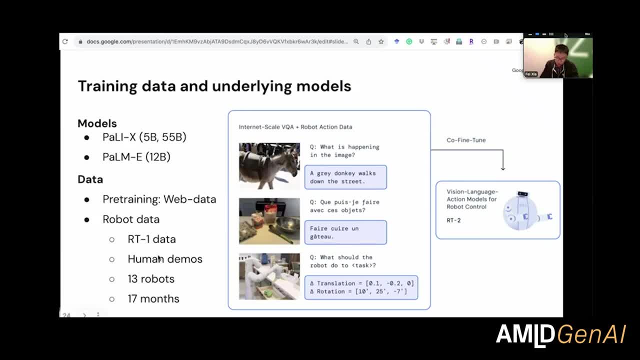 So all of these are human demonstrations. They are very difficult to collect And it's definitely possible to use reinforcement learning. We have been exploring similar directions. So in the beginning of the lab work there is QT-Op, which is using reinforcement learning. 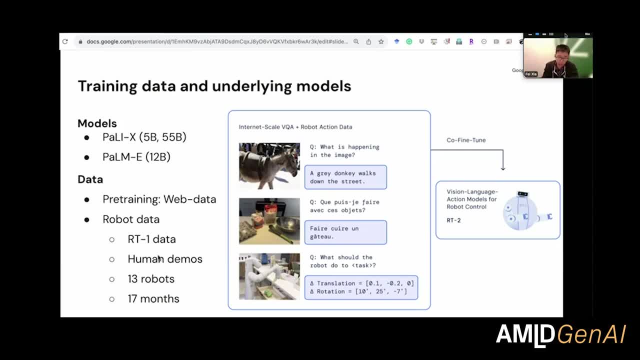 And we might have some follow-up on that regard. And I also want to mention that after you train this, you essentially get very good motion priors right, Because visual language model can give you a lot of prior knowledge of the world, So you might also 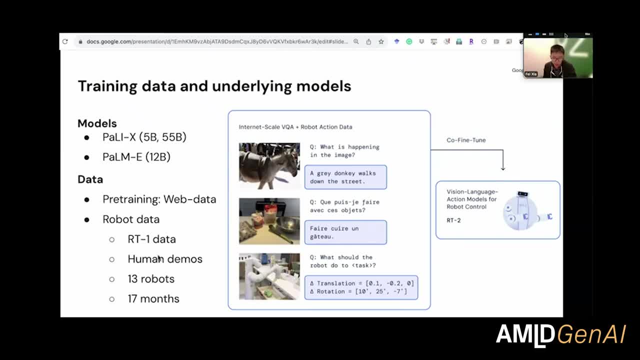 be able to use this as an exploration policy, And it's going to be a quite good exploration policy because it has a lot of understanding of the world And it also understands the development locus. And that's not all: We also have a temperature sample. 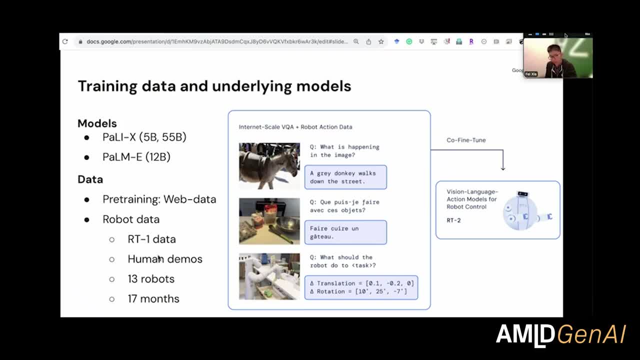 of those large-dimensional models So you can have diversity in your exploration, Like you might be able to do really good exploration with these robot-transformer models. One question: Can you do learning from demonstration or mutation learning by putting the human demonstration?